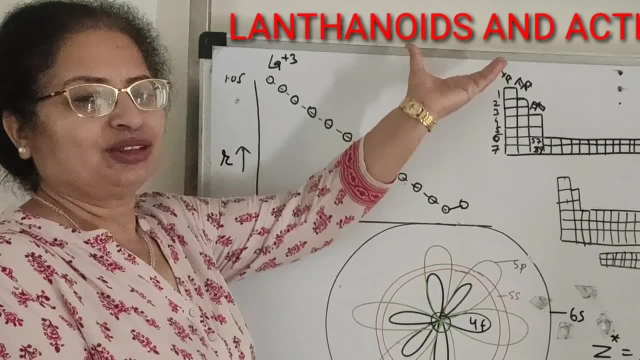 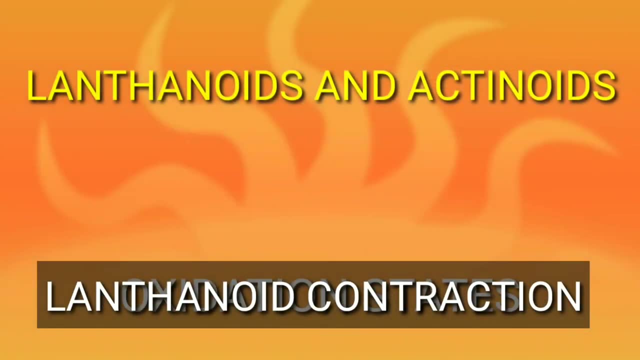 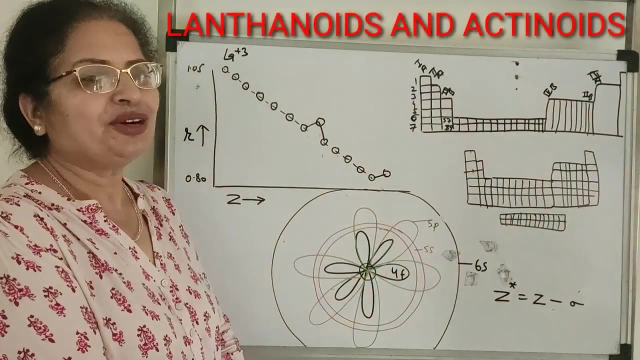 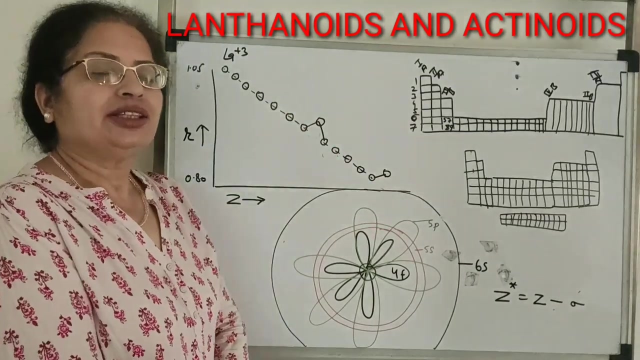 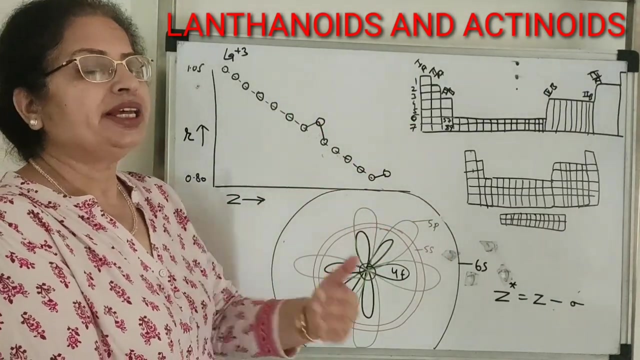 Hello friends, welcome to my channel. I am Dr B Narcitti, Associate Professor in Chemistry, and my today's topic is lanthenoid and actinoids. Lanthenoids and actinoids may. today we will discuss lanthenoid contraction. Before studying lanthenoid contraction, let me tell you that 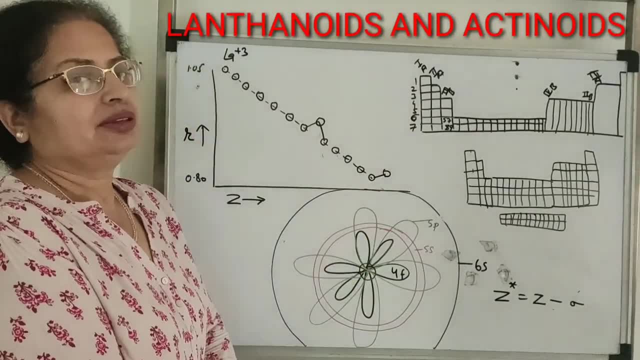 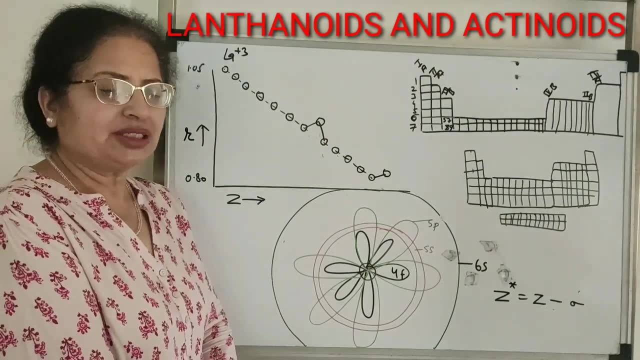 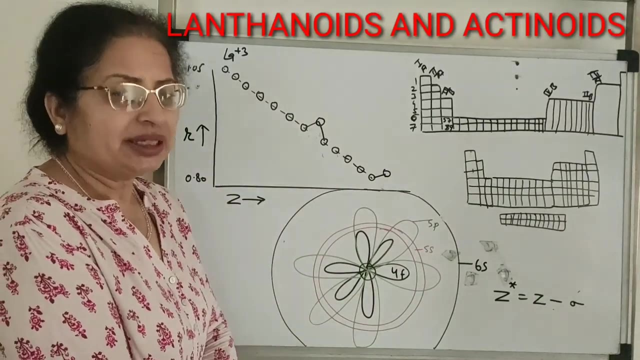 I have uploaded 2-3 videos on this topic in which I have discussed electronic configuration, oxidation states, magnetic properties and spectral properties. So I will recommend you to watch them first so that you can have a better understanding of these topics. So in 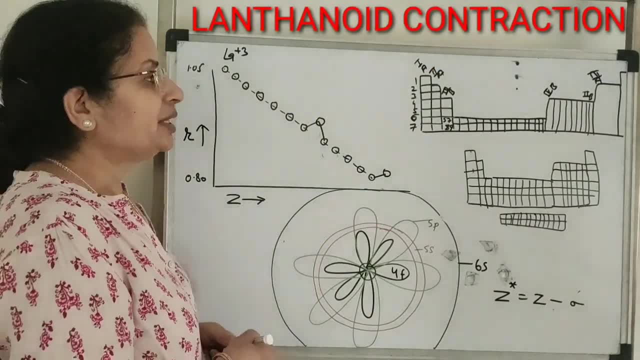 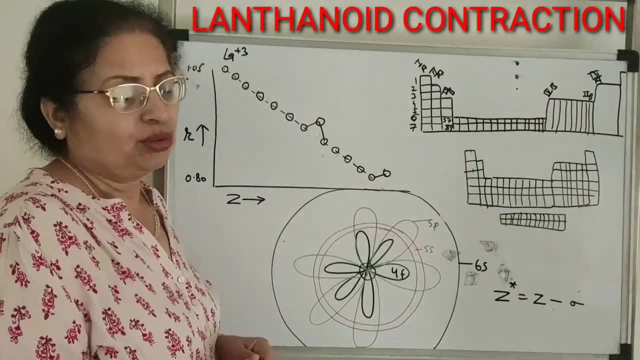 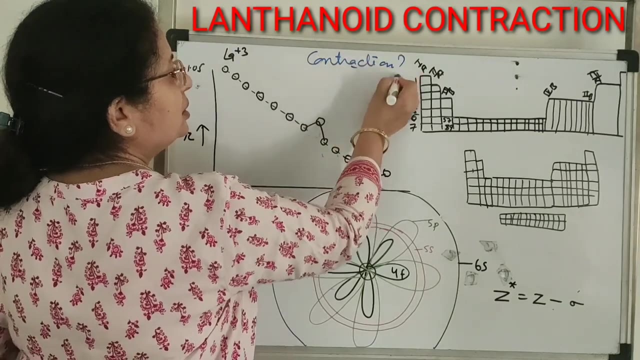 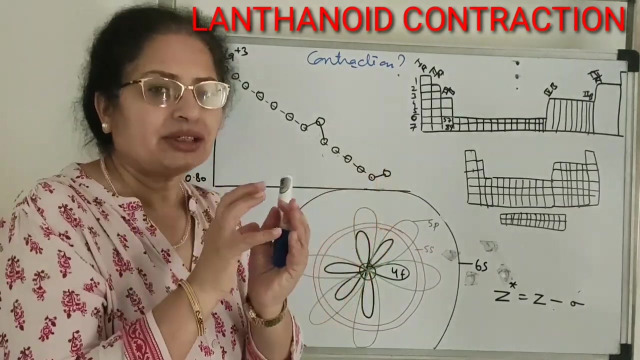 this topic, lanthenoid contraction. we will see that throughout the series, lanthenoid series size decreases. Why In lanthenoid contraction, the word contraction what does it mean? Contraction means shrinkage, ie contraction towards the inside shrinkage. 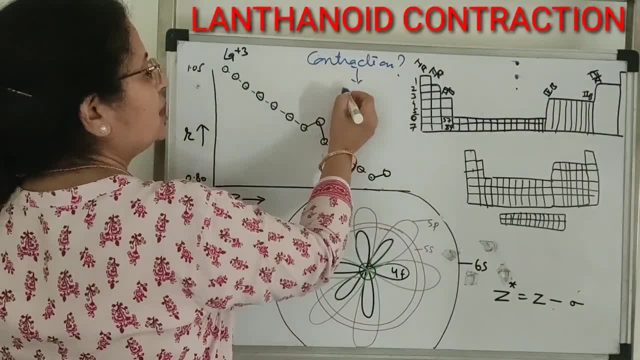 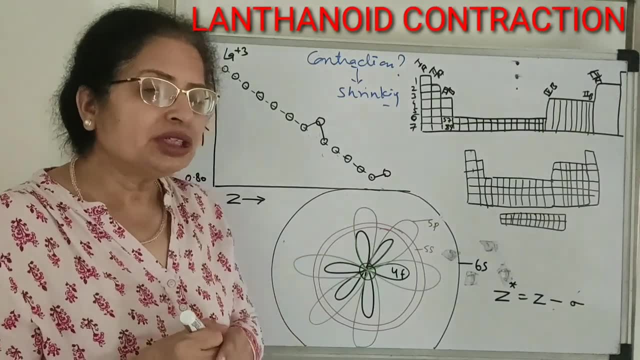 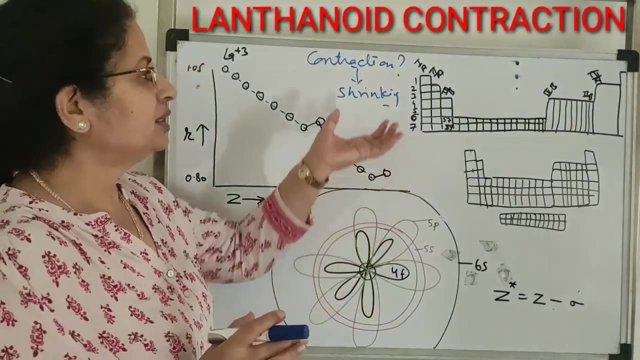 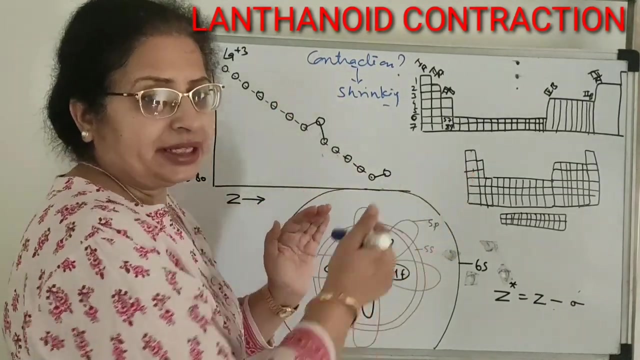 towards the inside of the shells. You can say contraction means shrinking, ie shrinking towards the inside, And lanthenoid contraction means that in the lanthenoid series the orbitals are shrinking towards the inside, So that is what we call lanthenoid contraction. Now let us read lanthenoid contraction Before. 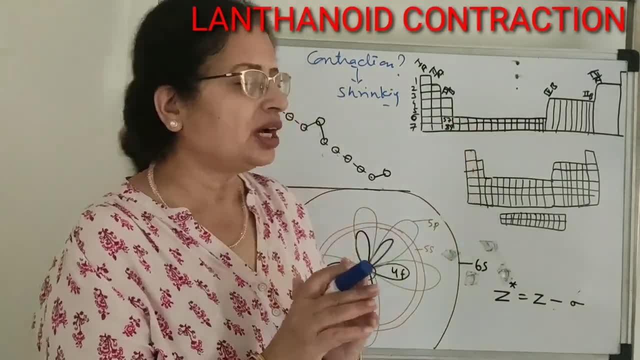 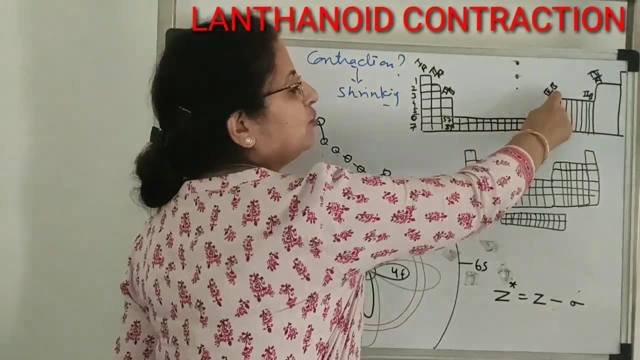 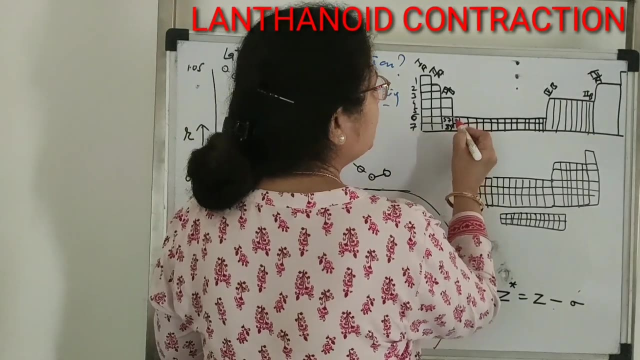 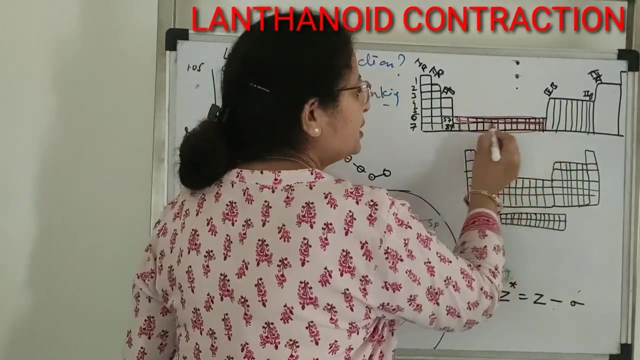 we see that. where is the position of the lanthenoid series? The position of the lanthenoid series is in the 6th period between 3rd B and 4th B. These elements that I have made, what do they represent? The lanthenoids, And what do the ones below it represent The actinoids? 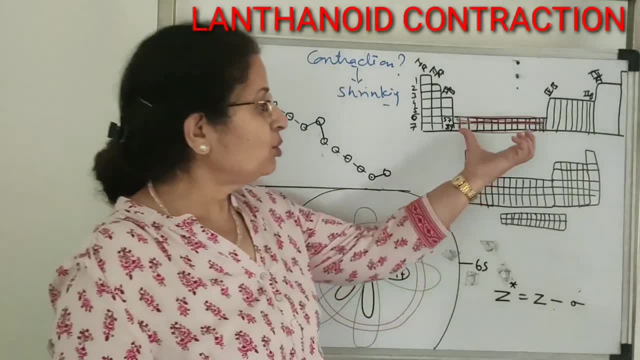 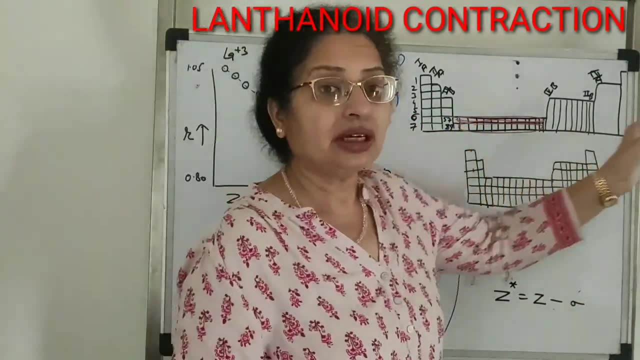 But I had told you earlier that because if we keep them here then the size of the periodic table becomes very big And there is a total size of the periodic table. So if we put them here, then the size of the periodic table becomes very big And there is a total size. 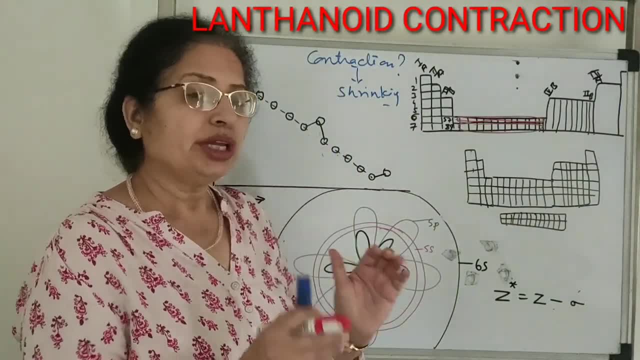 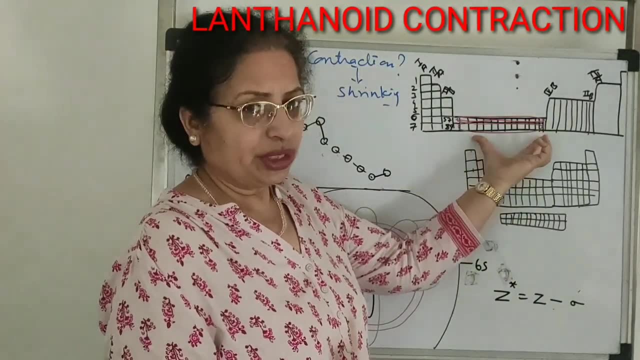 of the periodic table And the size of the periodic table becomes very big And there is a total size of the periodic table. So the class is 32 groups And it is difficult to print these 32 groups on two pages. So we take these 14 groups and put them under this And 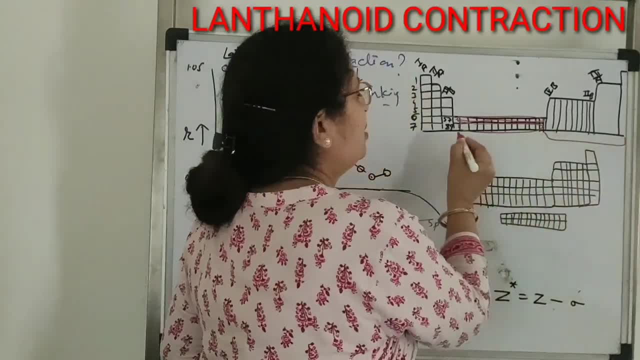 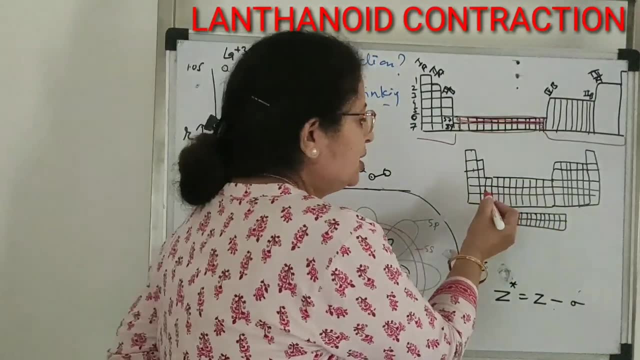 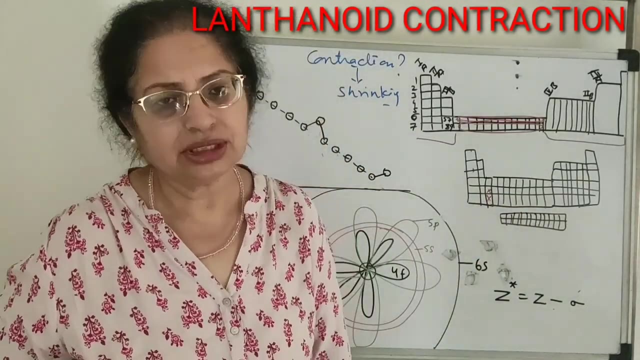 these the parts of the periodic table. these parts and these parts we make them as clubs and we get this new periodic table And in this we put two stars here that represent that the lengthenoid and actinoid series starts from here. 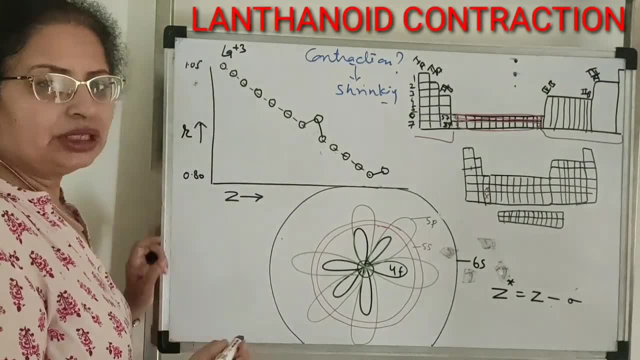 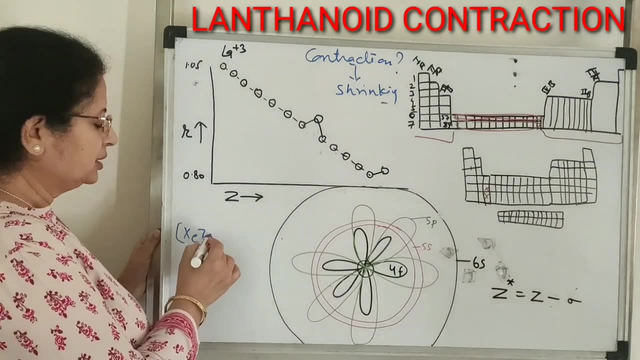 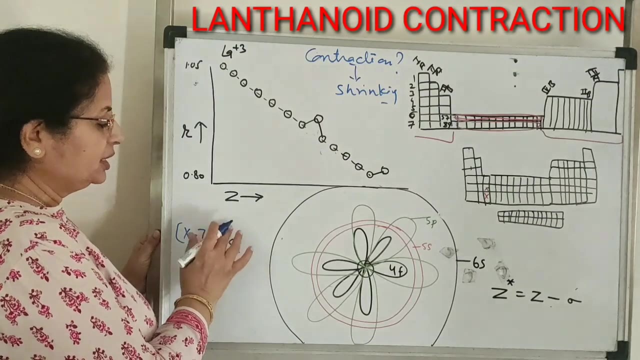 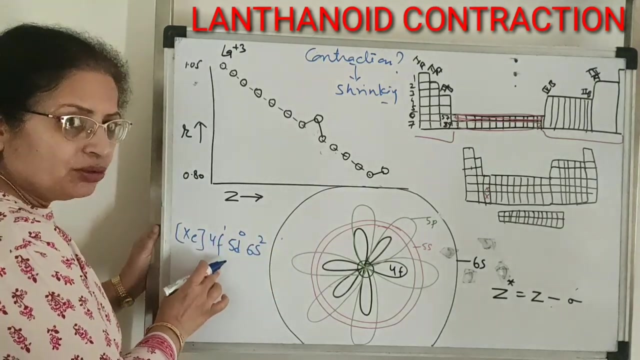 If we see its electronic configuration of lengthenum, then it comes here. xenon after xenon comes your 4F1 and along with it comes 5D0 and 6S2.. It should be like this, but because it does not follow the principle, 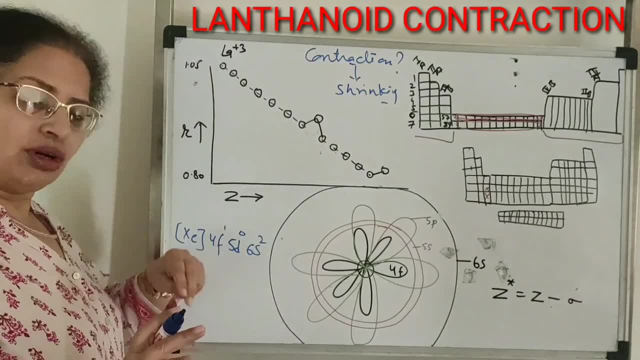 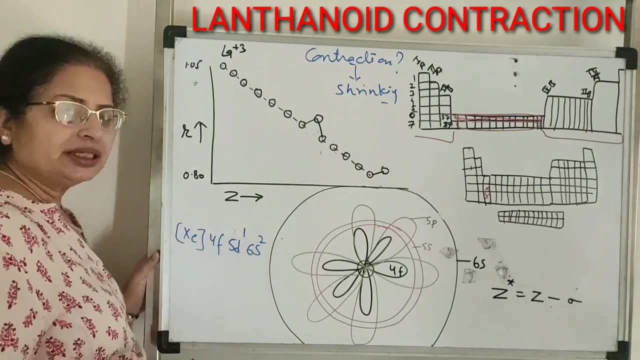 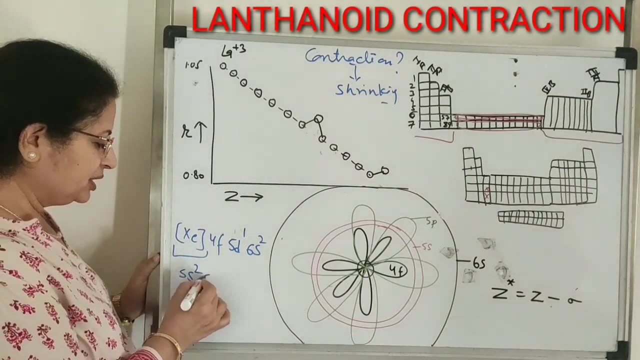 and it has more energy of 4F, which we already have discussed in my last video. so that is why its electron does not go to 4F, but enters 5D, And if we see xenon also, then its last configuration comes 5S2, 5B6. 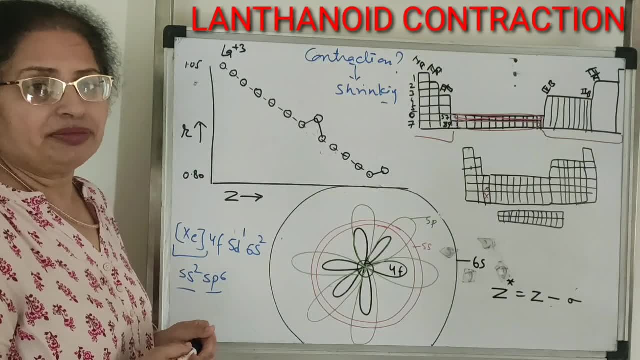 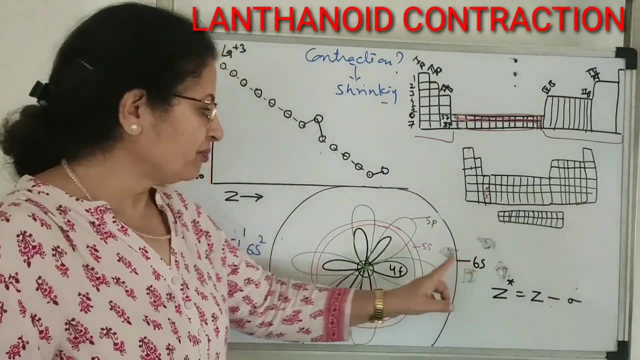 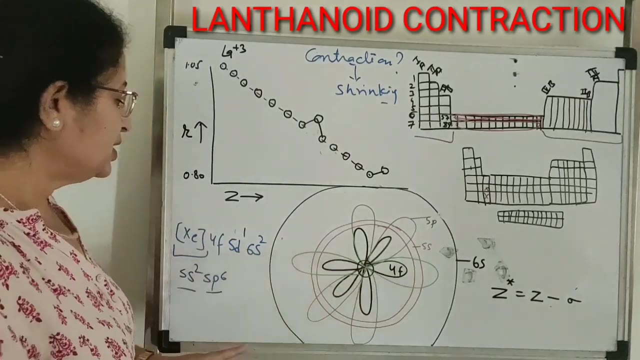 This means that lengthenum serium presidium, in all these cases, which is going to be the outermost shell is 6S, Then which will be inside it 5S and 5P. Here I have drawn 5P and here I have drawn 5S. 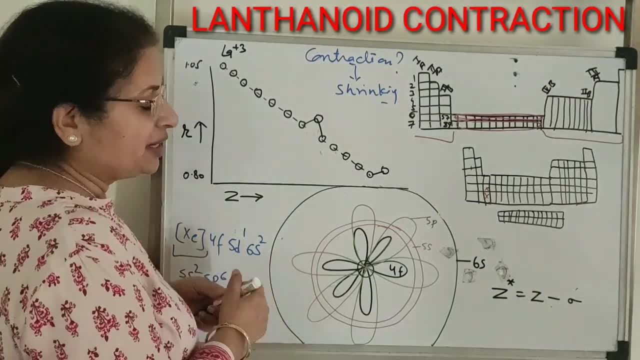 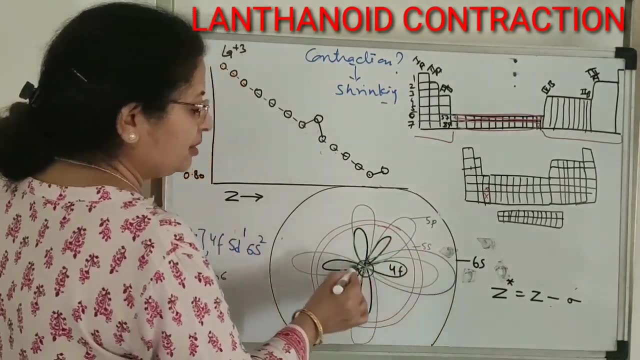 After this comes 5D. Where will 5D be? If this is 5S and this is 5P, then where is 5D going to be? It is also going to be outside, So I have decided 5D. 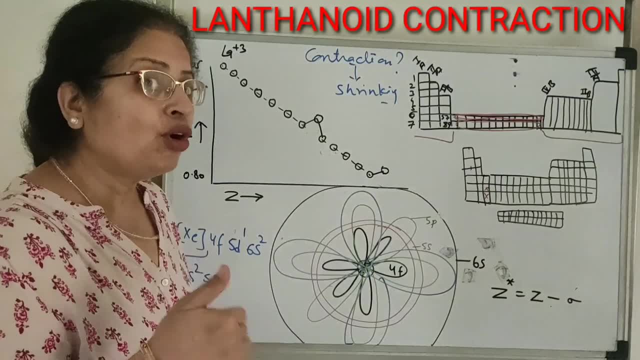 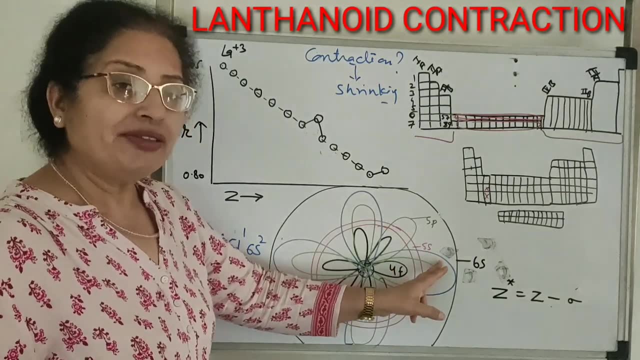 I have drawn 5D. Now tell me, where will 4F be? Neither in this outermost shell 6S nor in this 5S, 5P, 5D. but it is also inside it What I have drawn from the inside with black colour. 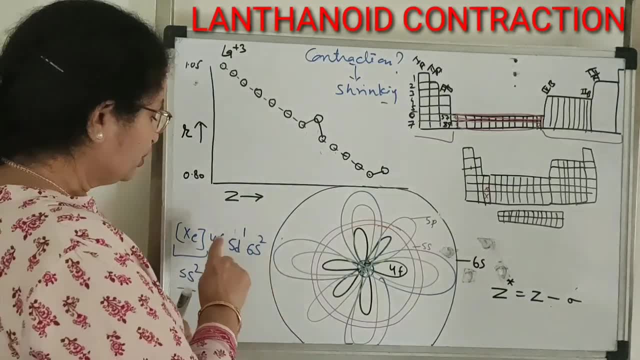 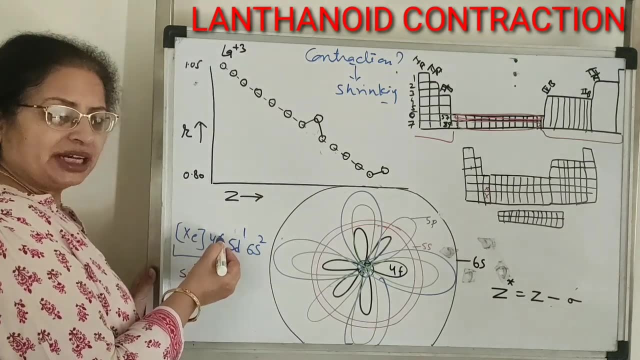 what is this 4F orbital? So where do all our coming electrons go? Because in 58, it jumps to this electron and comes here, And then it becomes 2,, then slowly 3,, 4,, 5,, 6,. 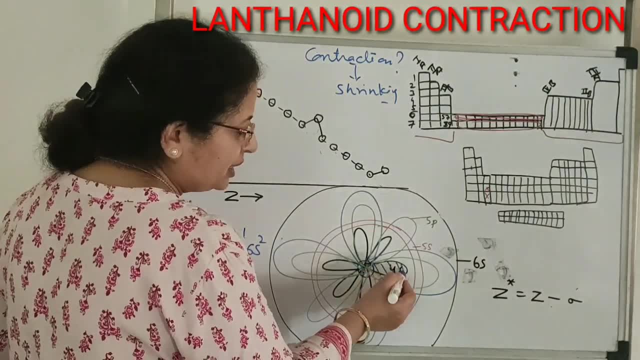 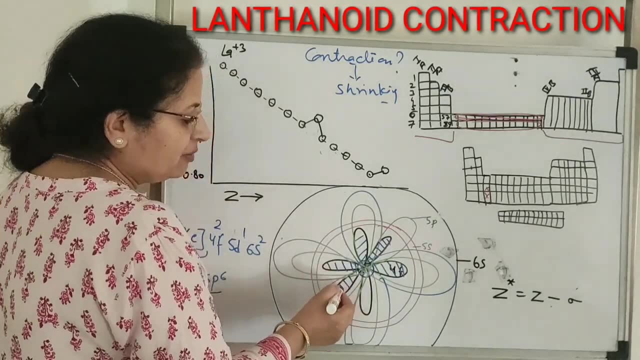 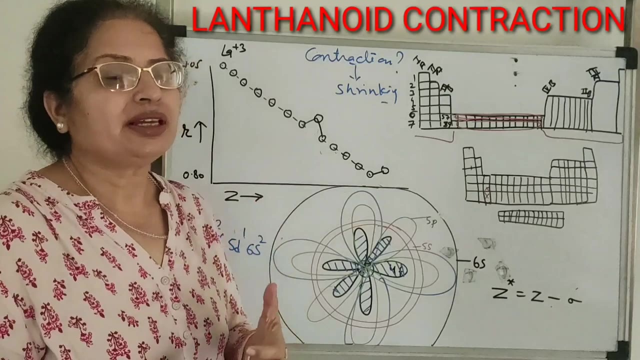 likewise, it increases to 14.. Means the electrons which are going to come to 14, where are they going to come? They are going to come in these 4F orbitals, But what are we seeing? The protons are also increasing. 57,, 58,, 59. Where are they increasing Here? Here In Z, Increasing in the nucleus: 57,, 58,, 59,, 60. Increasing in this way. So what does the atomic size depend on? 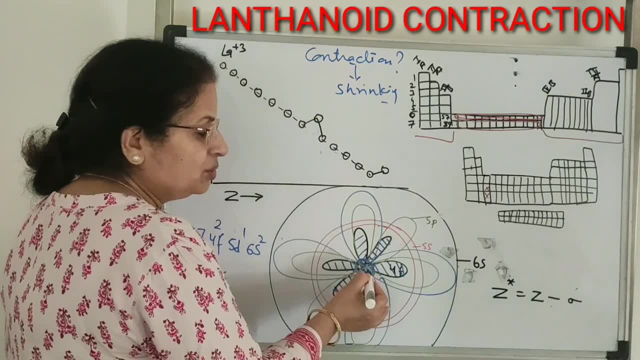 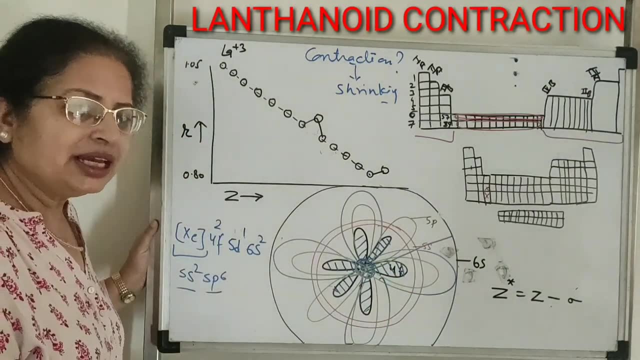 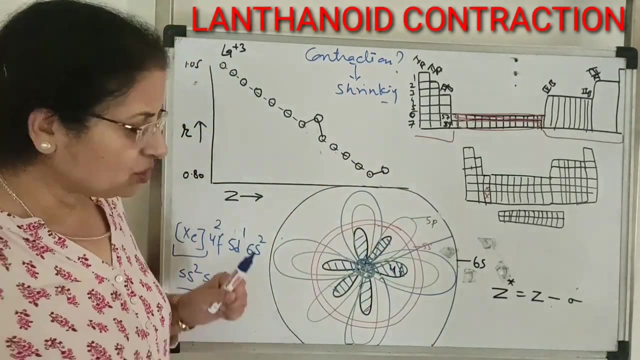 If this is the outermost shell and this is the nucleus, then the distance between the nucleus and the outermost shell, what is it called Atomic radius? And if we make an ion in it, that is superb. let's say what? 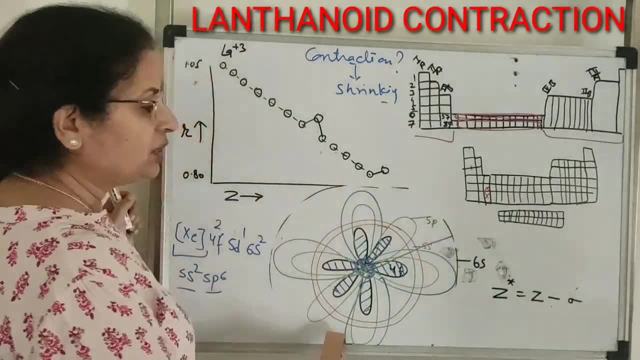 Atomic radius. вам个 pero dáng. So take the distance upto 5.. The distance between the nucleus and the outermost shell, The atomic radius In an ót эта, extends in the atom to 5.. I'll tell you about an atom. 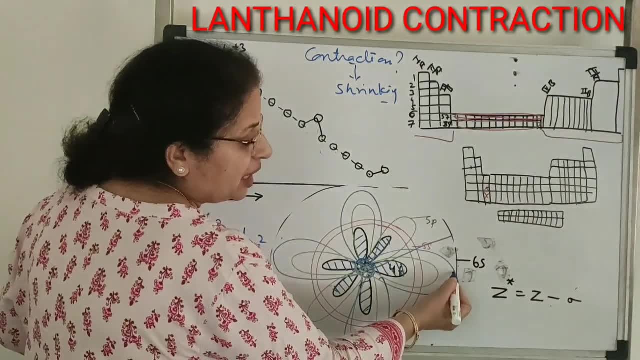 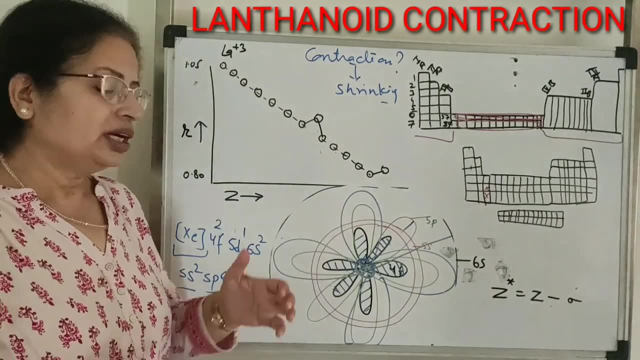 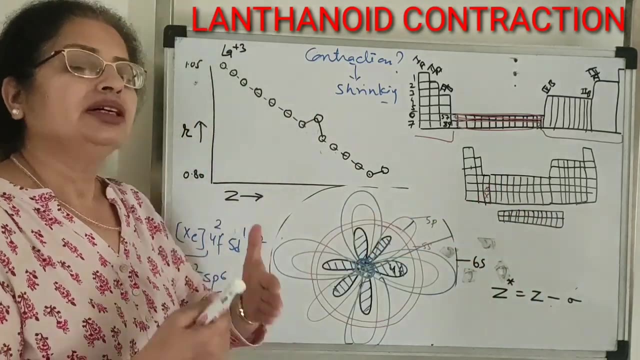 So, we'll think of an atomic-radius. This distance paris, or seems to be the other way round. This redundant electron. This basic electron is Jacobian, if it is vou de 6 second. This electron would change into dad or we take the � None, 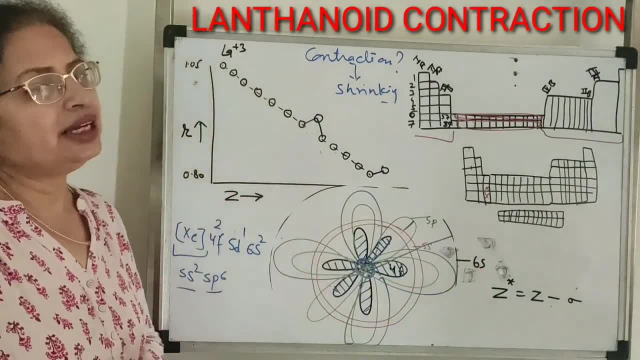 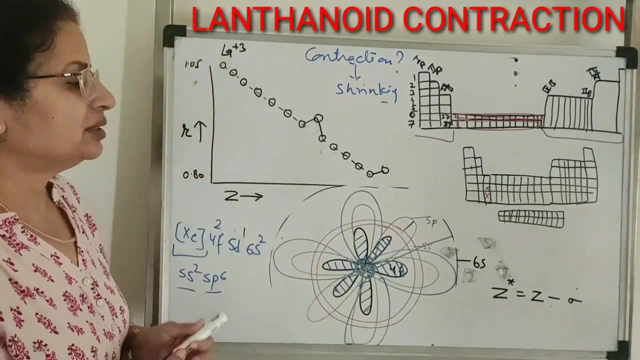 out and the distance between the outer most shell is called ionic radius. So here we are looking at ionic radius, and if we make atoms, then we are looking at atomic radius. So which factor will that atomic radius depend on? It will depend on two factors. 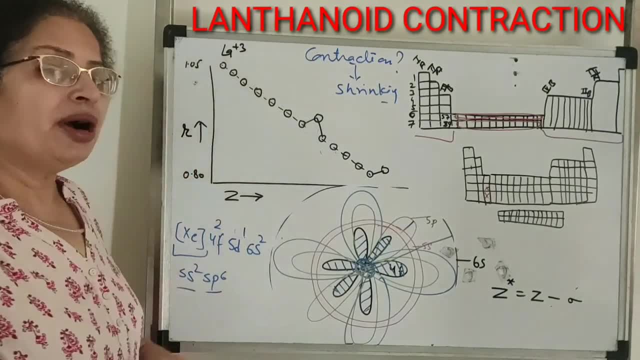 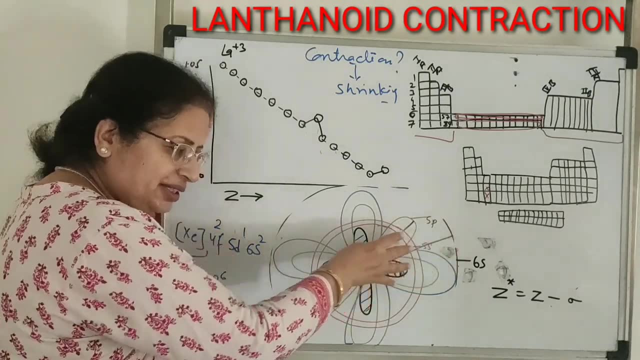 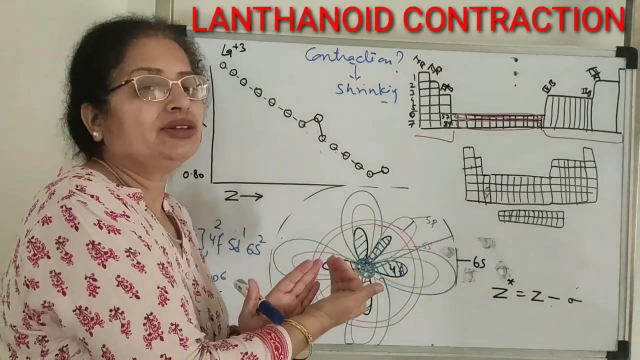 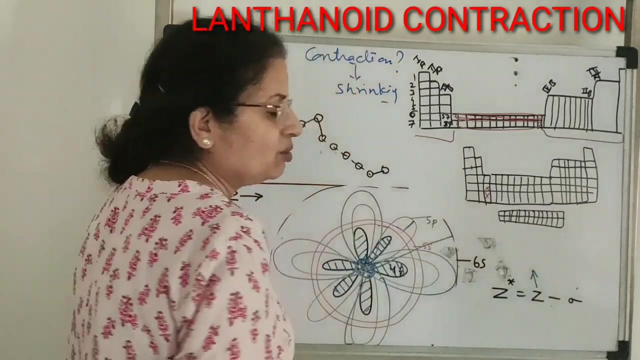 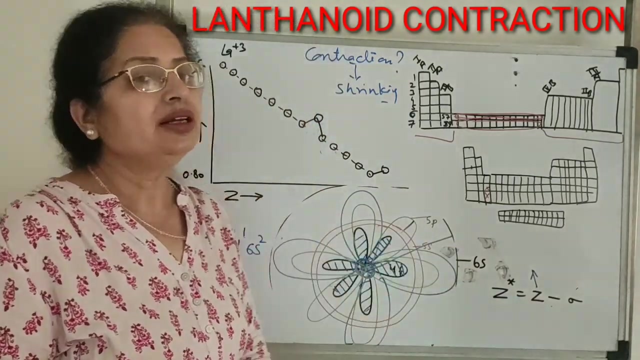 That is Z and sigma meaning shading effect. Z is nuclear charge. This nuclear charge attracts the electrons of minus to the inner side so that all these shells contract inside and shrink. So as Z increases, size will decrease because of contraction. But there is another factor which we call sigma. 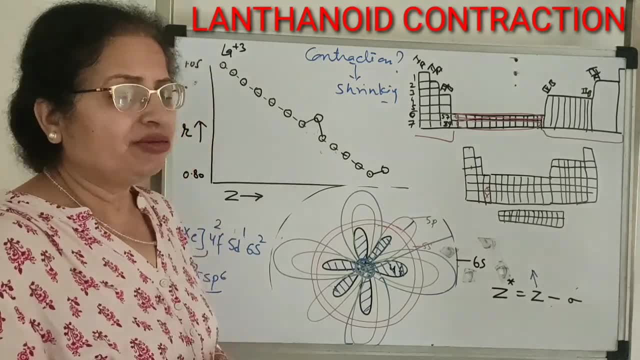 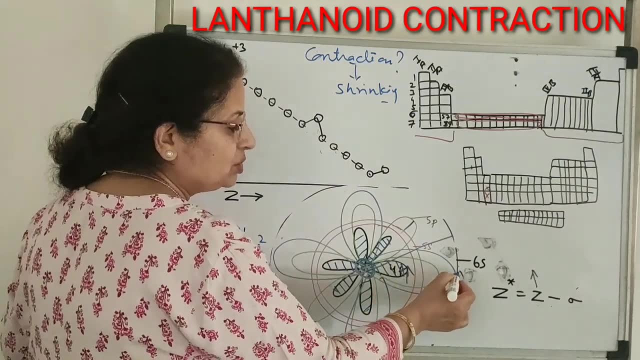 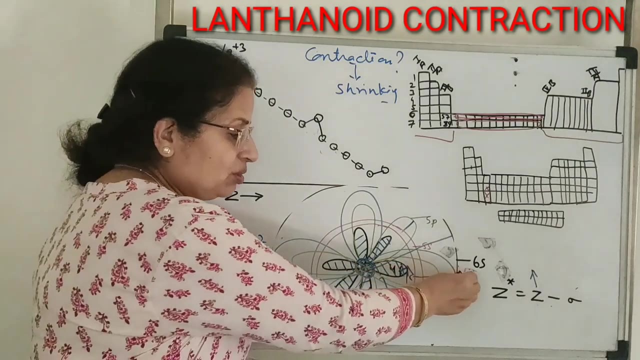 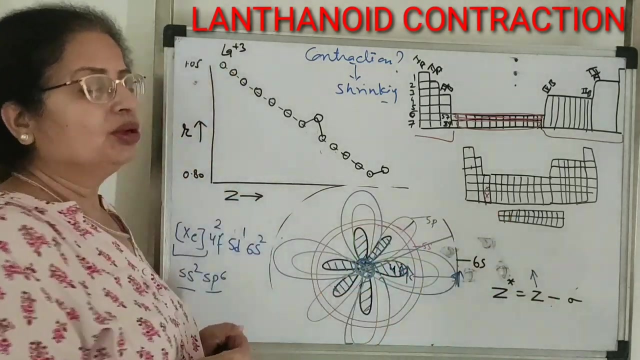 Sigma means shielding effect. What is shielding effect? Shielding effect is the repulsion between the inner electrons and the outer electrons, because they are of minus to the minus side. So as the nucleus asks the electrons of this shell to come inside and these electrons of 4F ask them to go out, 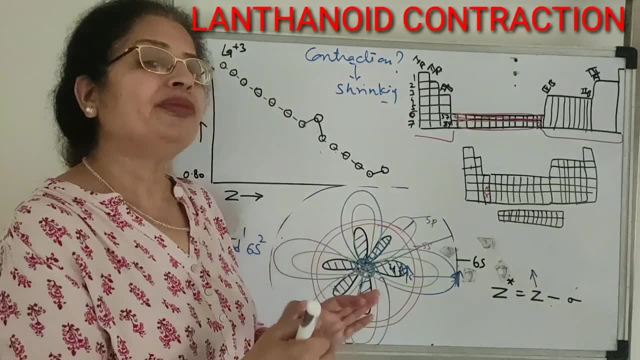 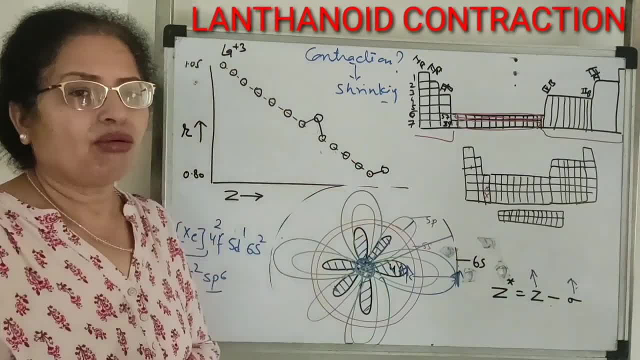 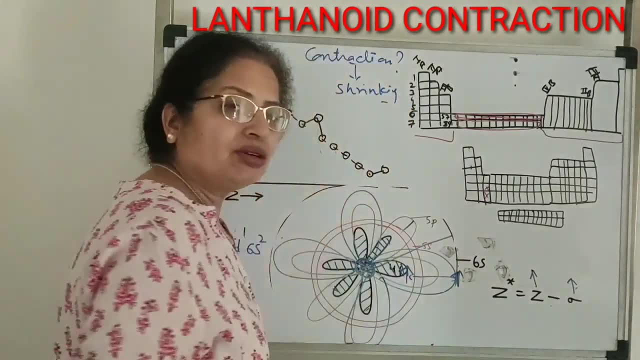 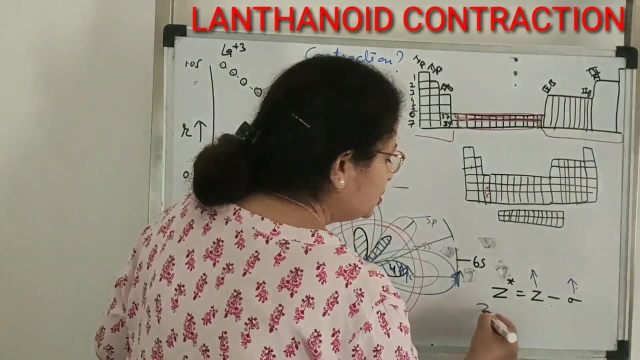 Sigma is expansion. So what will happen to net? Net will depend on Z star, That is, who is dominating out of these two? That is Z star, we call effective nuclear charge. We will also show this with Z-effective Effective nuclear charge. 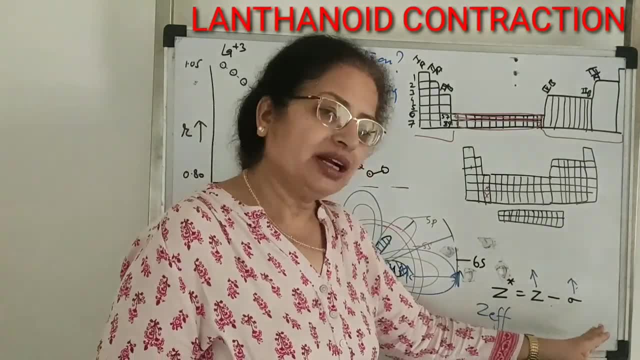 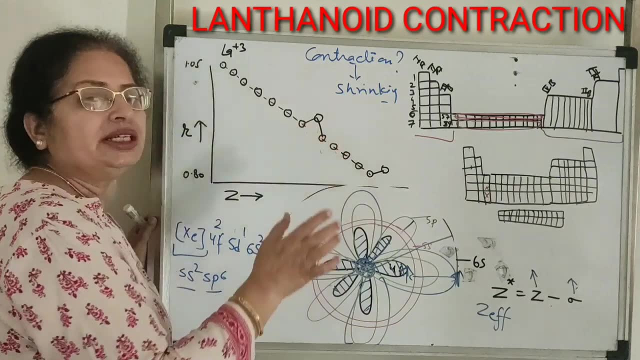 So what will be the effective nuclear charge If we minus the shielding effect from Z? So now we will see that how much is the shielding effect of these F-orbitals? So I will tell you a little bit of the old class, which is the Slater's rule. 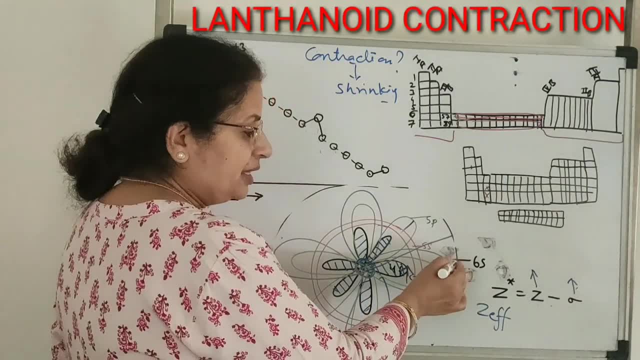 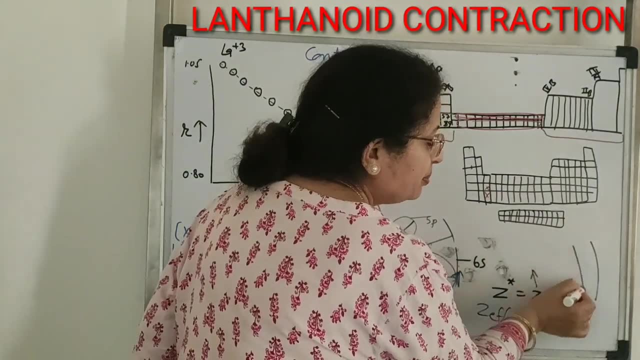 Slater's rule says that if the electrons on the inside are in S-orbital See, this is the outermost, this is the penultimate and this is the antepenultimate. So we will discuss how much repulsion the outermost electron is getting. So the repulsion of the outermost electrons is less, But the penultimate of its inner shells is approximately 0.5.. So we get 80%, which we consider to be equal to 0.8 proton, But the penultimate of the antepenultimate is also in S-orbital. 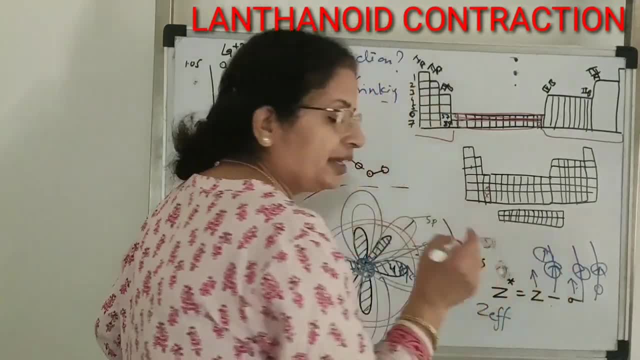 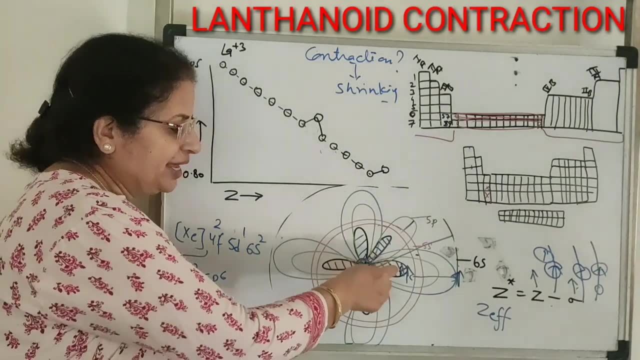 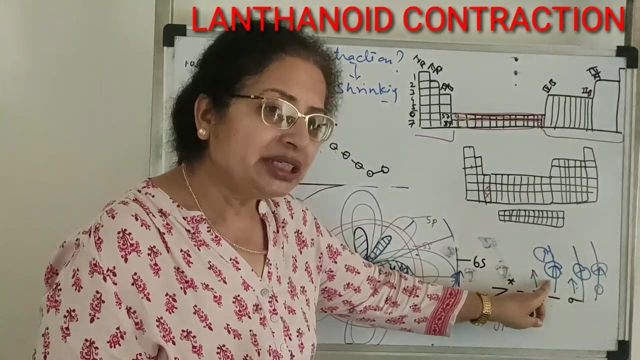 So it is equal to 1.. So one electron cancels the charge of one proton. Z says: come inside. So what does this one electron do? It sends it out completely. But this happens when the electron of this penultimate shell. In which Either in S-orbital or in P-orbital. So if we increase the electrons in S or P-orbital in the penultimate shell, So what will happen? Size will not be affected. Why? Because Z is increasing by 1 and shading effect is also increasing by 1.. 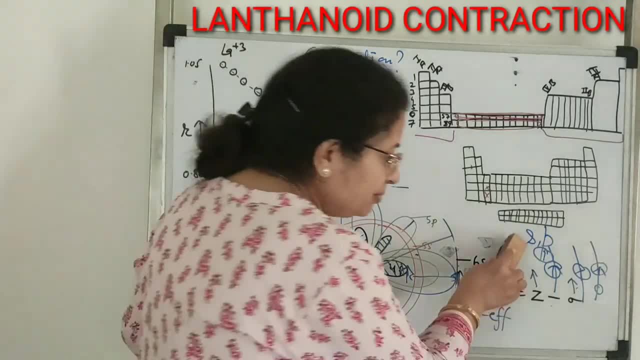 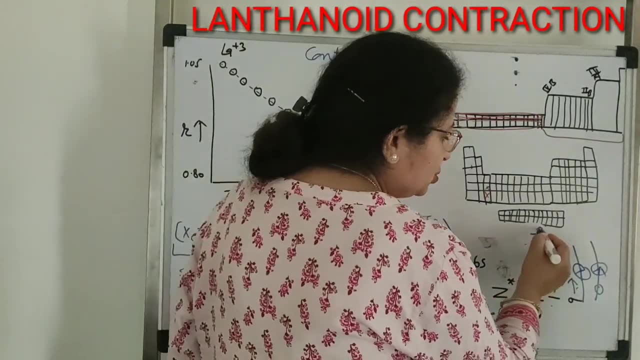 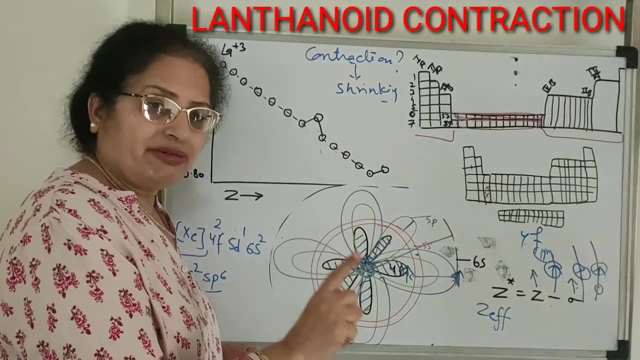 Now, what are we actually doing? Our antepenultimate shell, This outermost penultimate or antepenultimate shell, In which orbital are we filling In? 4F? Its shielding effect is not equal to 1.. Now, what happens if it is not? 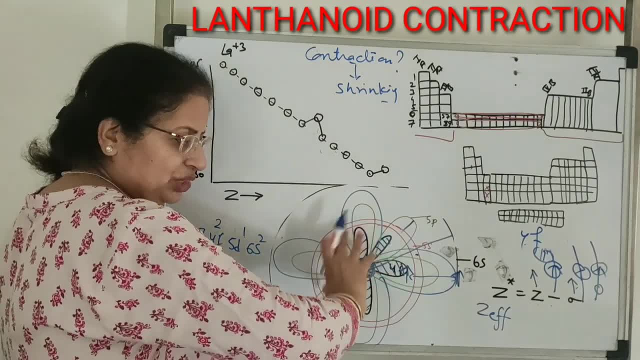 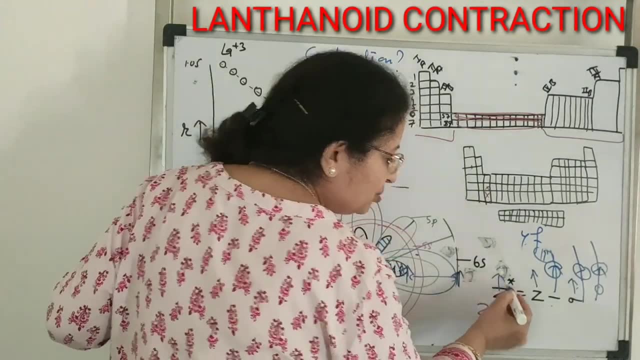 That means it is not able to shield it equal to 1 proton. So what will happen? Net nuclear charge will increase. And when the net nuclear charge increases- See if this increases by 1 and this increases by 1. Then this does not increase. 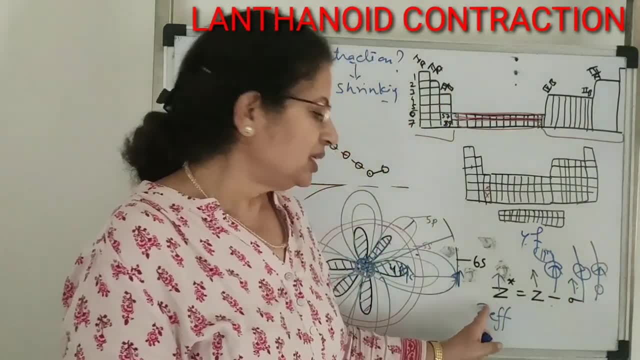 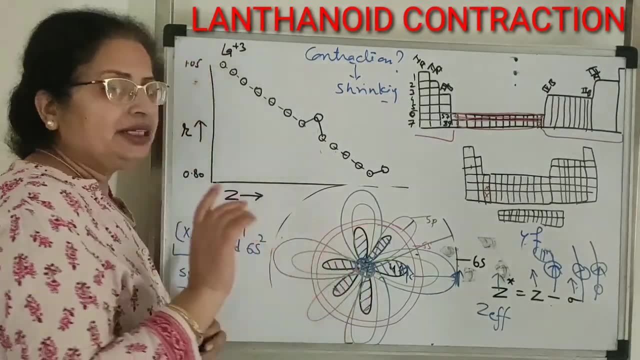 But now this increases by 1 and this increases by less than 1.. So what is Z-effective? It increases. So here comes the first factor. What is the shielding effect of this 4F orbital Less? This does not cover the whole nucleus. 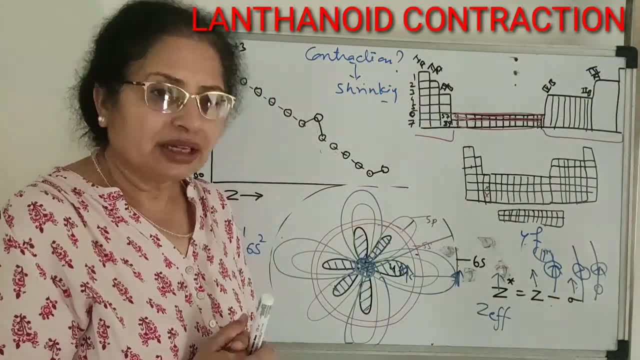 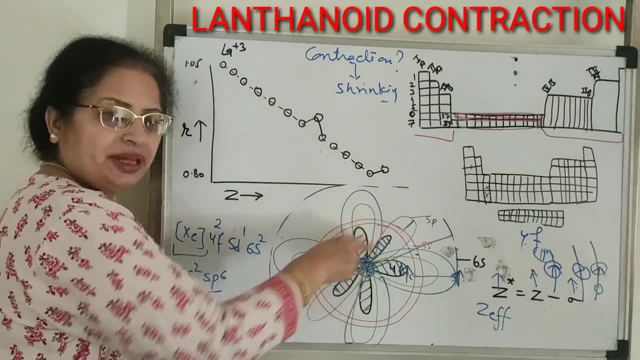 And secondly, what is the repulsion from here to here? Less Why? Because it is dispersed. There is no concentrate in one place. One electron is going in 6 directions. So what does this mean? It is empty from 5 sides. 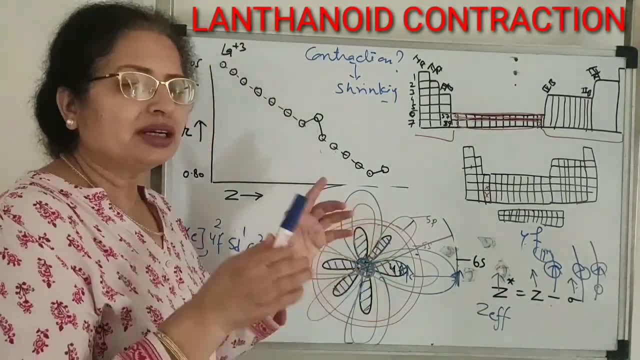 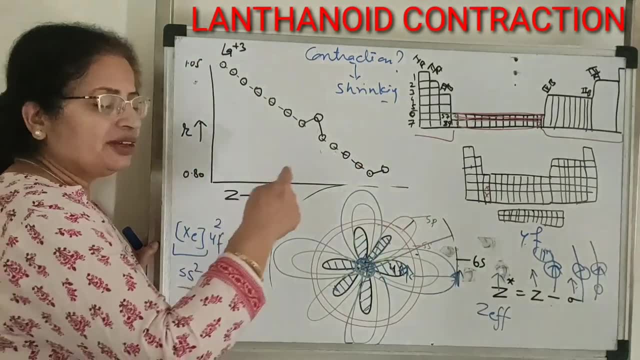 At a time, it will be in one place. So if its shielding effect is less, What is Z-effective? It increases. So when you go from 57 to 58,, 58 to 59, in this way, 57,, 58,, 59,, 60,, 61.. 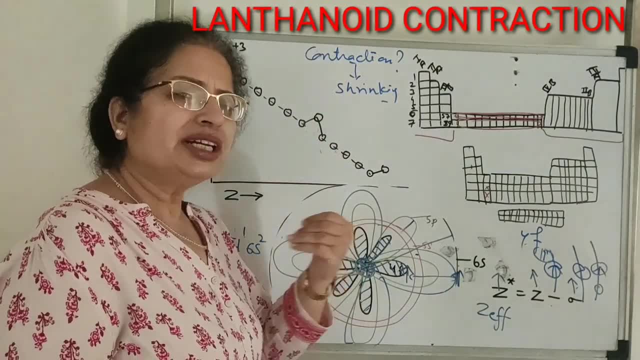 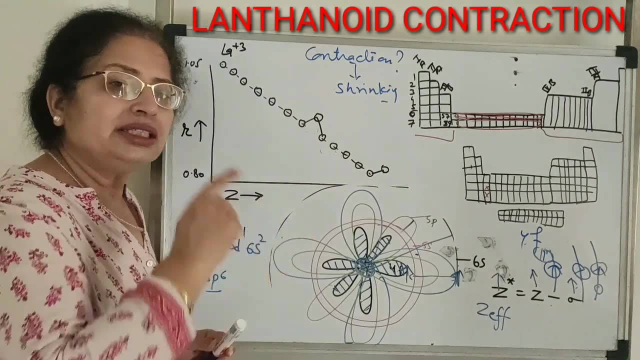 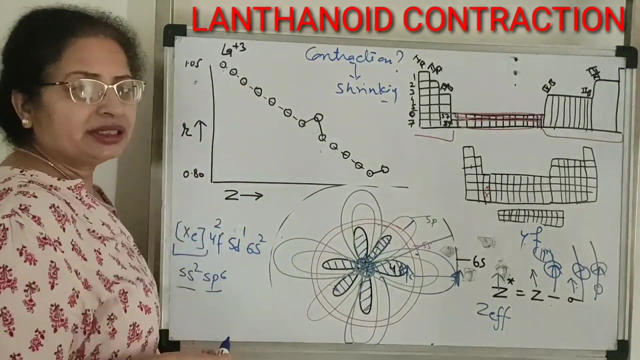 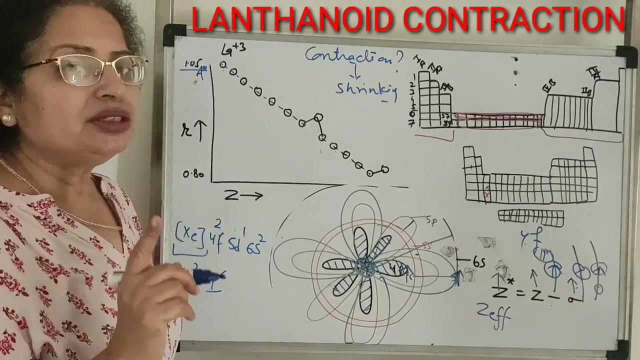 So the shells are inside contract regularly and gradually. Due to this, their size decreases And this decrease is called lanthinoid contraction. Now, if we see the size of the first element of lanthanum plus 3 ion, then it is almost equal to 1.05 extra. 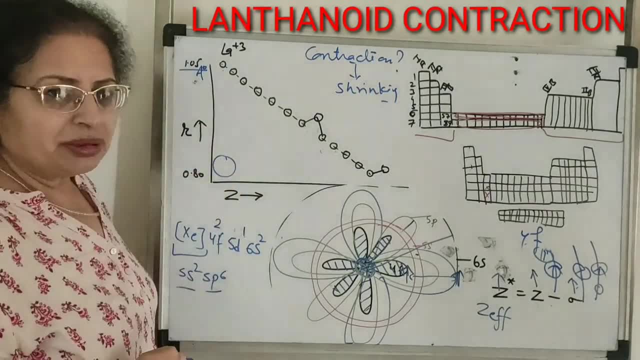 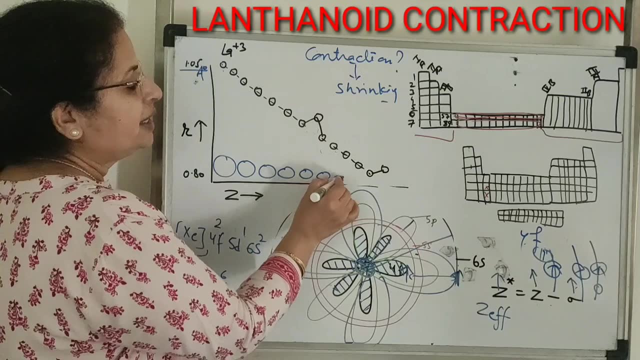 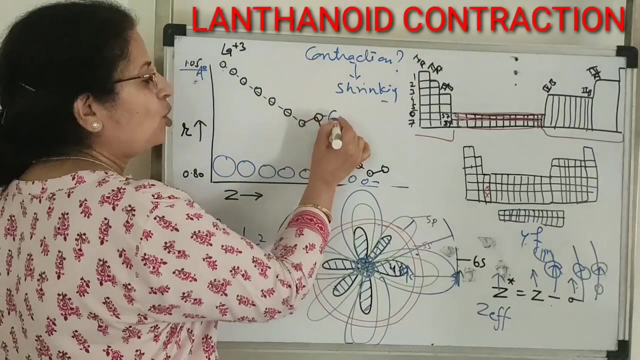 Means if it is this big, then as you move left to right then the size will gradually and regularly it will decrease. But here in the center, in the middle of the series, in the case of European plus 3,, F7 configuration happens. 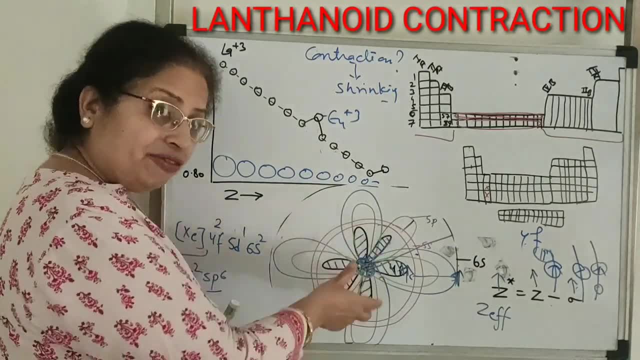 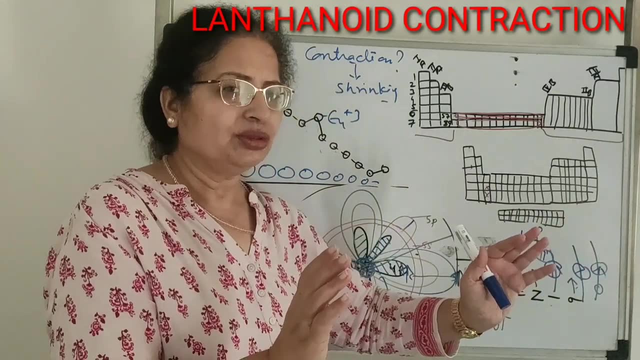 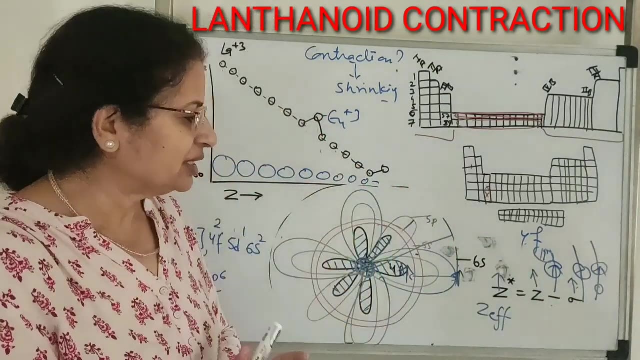 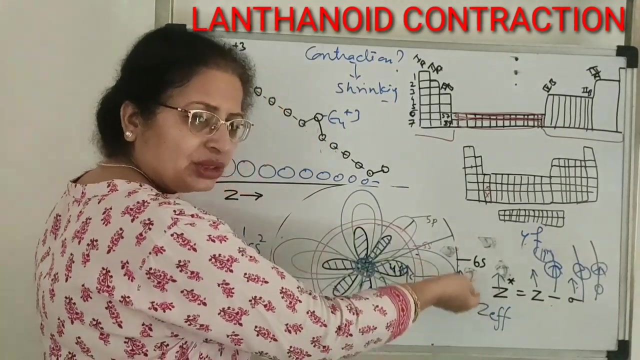 When F7 configuration happens, then it means half-field configuration. If there is a half-field configuration, then the shielding effect increases a little more because the orbitals are in full tension, in full size and they cover the nucleus a little more. So that's why the shielding effect increases here. the effective nuclear charge does not increase that much, it increases a little less. So here the size increases a little, then it is regularly decreased. And what will happen in the last, As soon as you reach the lutetium, then what happens? there the size increases a little. Why increase? Because there the configuration comes F14,. F14 means full-field. 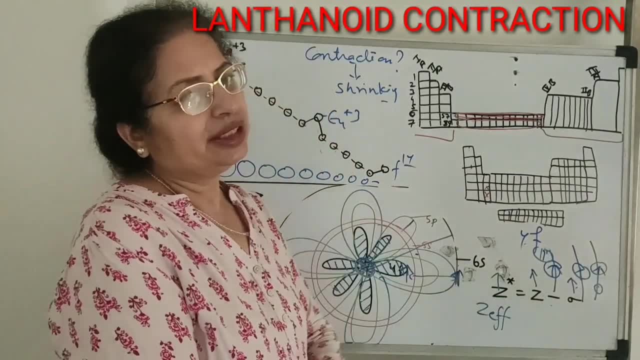 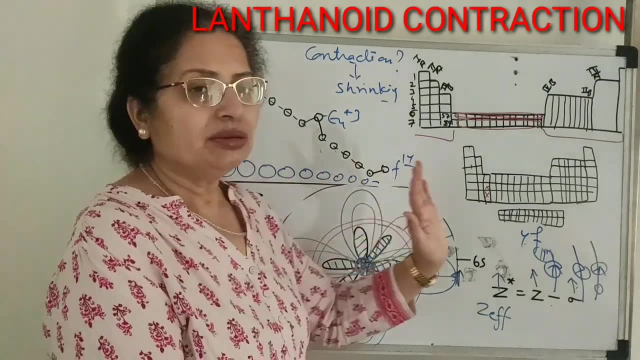 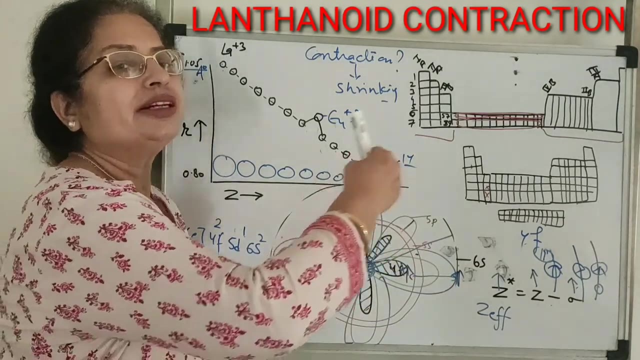 What is the shielding effect of full-field configuration? It is more. that is why the effective nuclear charge does not increase that much. So this was the lengthenoid contraction in the brief, That is, in the lengthenoid series, The gradual and regular contraction that is coming in the size that is called lengthenoid contraction. 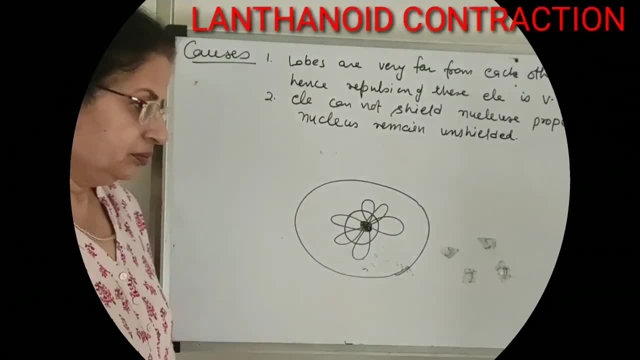 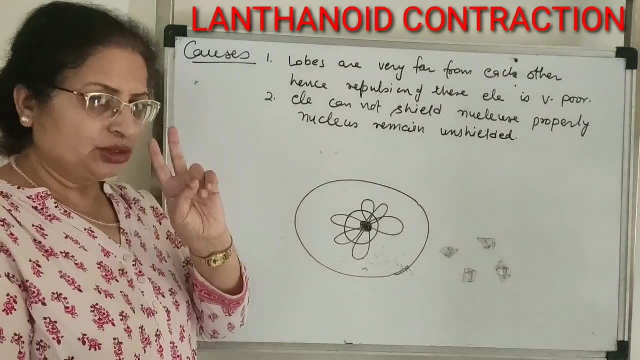 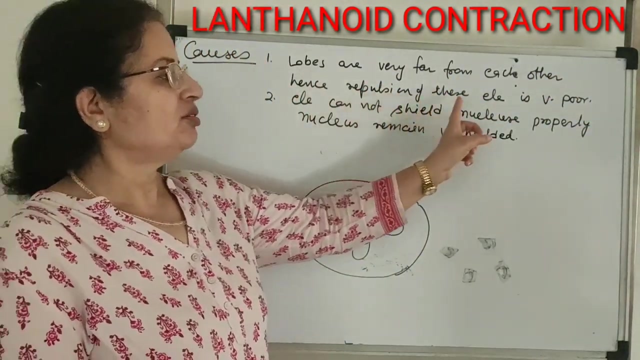 Now we will study its causes and consequences. Causes of lengthenoid contraction. In the causes of lengthenoid contraction there are two basic causes. First, the lobes are very far from each other, Hence repulsion of these electrons is very poor. 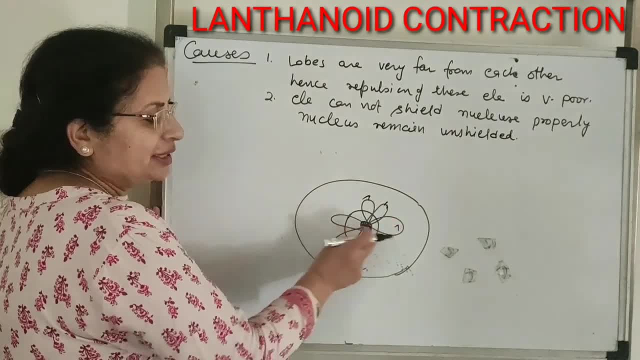 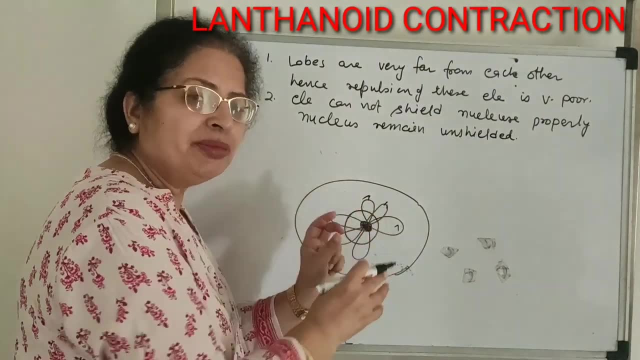 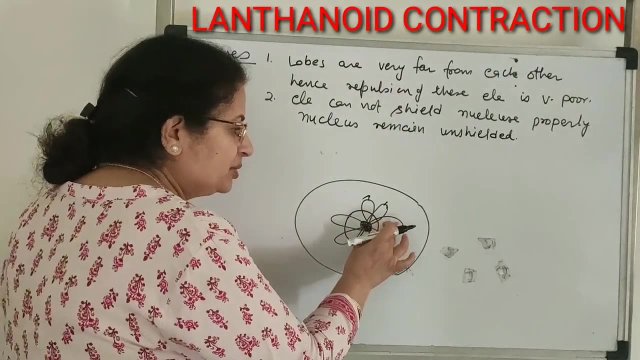 Because the lobes of these 4F electrons are very far from each other at a time. Because by combining these three lobes, by combining these three numbers, by combining these six lobes, what happens? One orbital is formed, And if there is one electron in it, then at a time it will be in one place only. 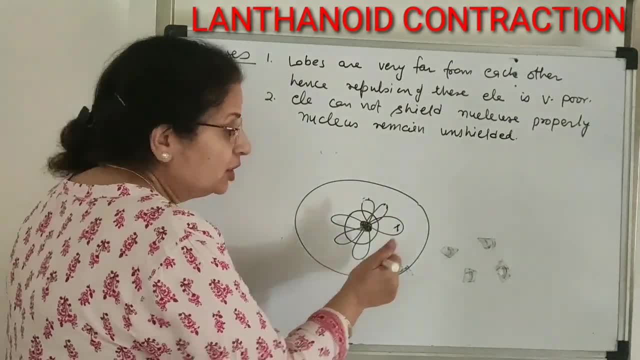 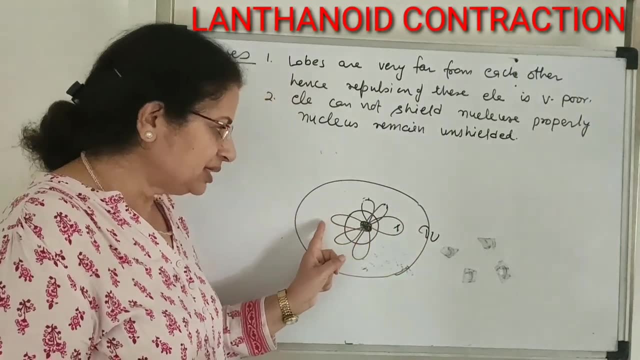 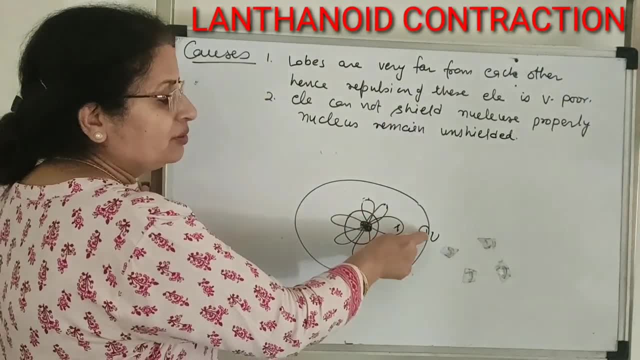 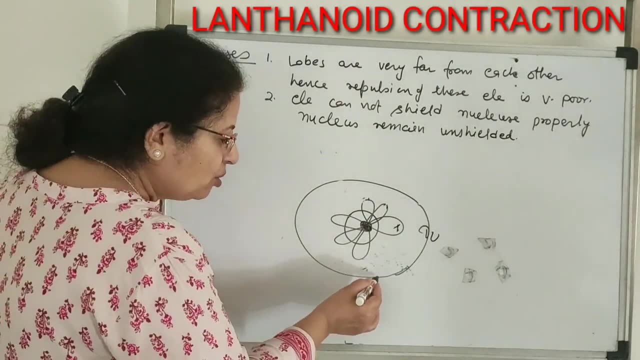 So what will be the consequence of this? When these electrons will reach here, here, here, here, here, then they will keep getting the attraction of the entire nucleus, And when they are here, then they will feel attraction towards the inside. 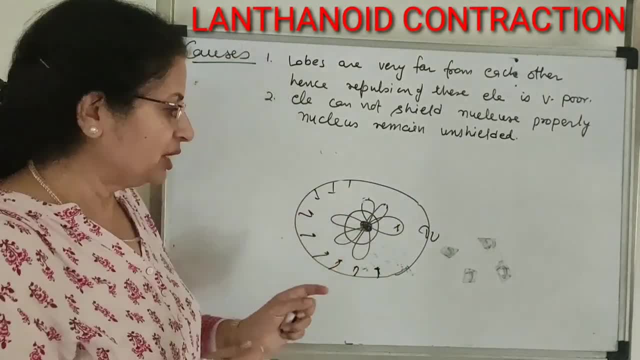 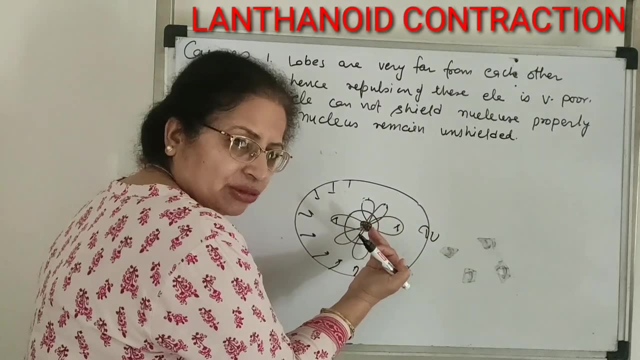 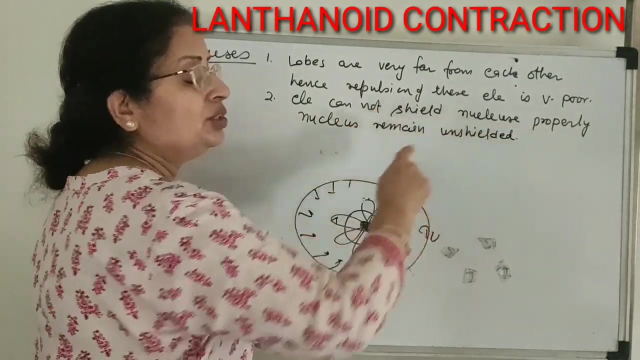 And what will happen? They will contract towards the inside. Now, when this electron will come here, then what will happen? This shell from this side will feel the contraction towards the inside. This is the first factor. Secondly, electrons cannot shield the nucleus properly. 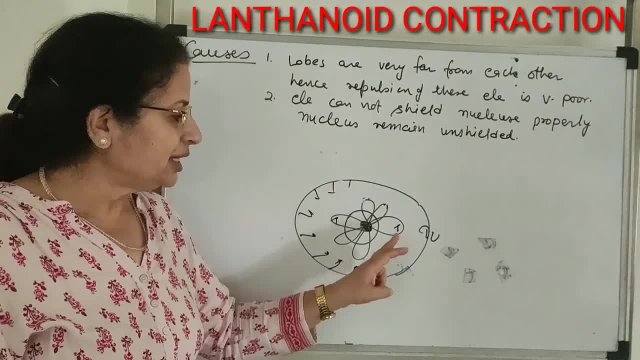 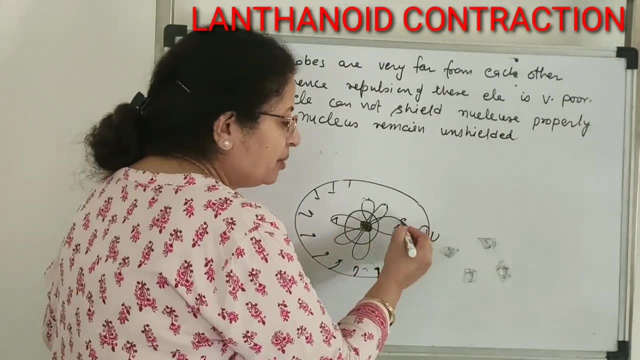 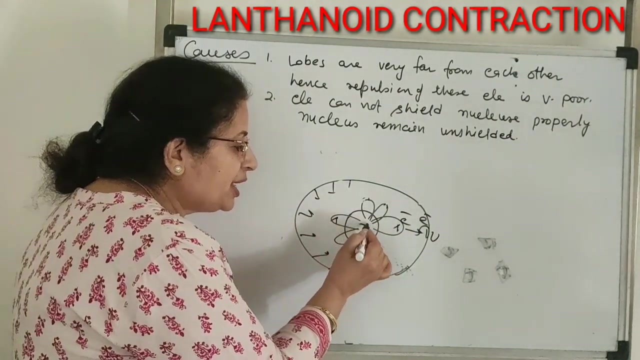 Nucleus remains unshielded, Because these electrons work in two ways. One is to repel the external electron due to minus minus. Secondly, this whole plus charge in the nucleus, this plus charge has to be protected by the minus. This is called shielding. 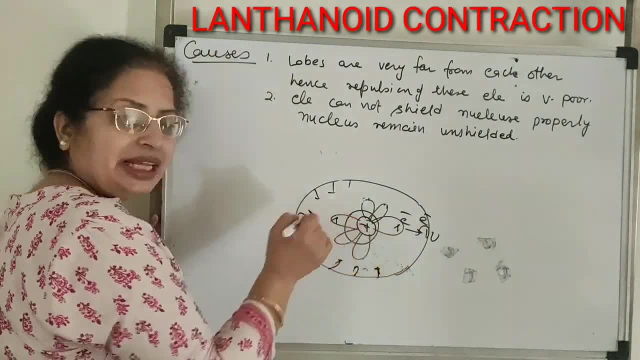 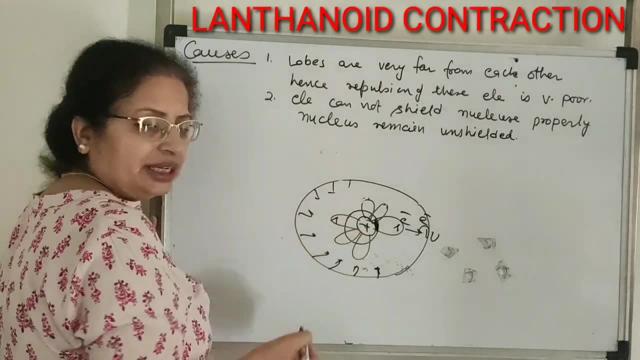 Shielding means covering it. So when it comes to covering it, then what will happen? If this electron is on this side, then what will it do to the nucleus? only from this direction It will shield it. What will happen from the rest of the side? 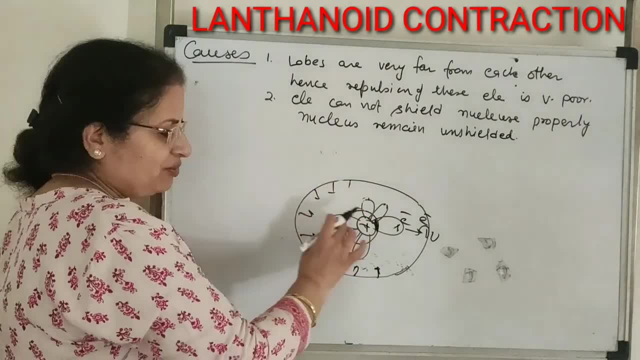 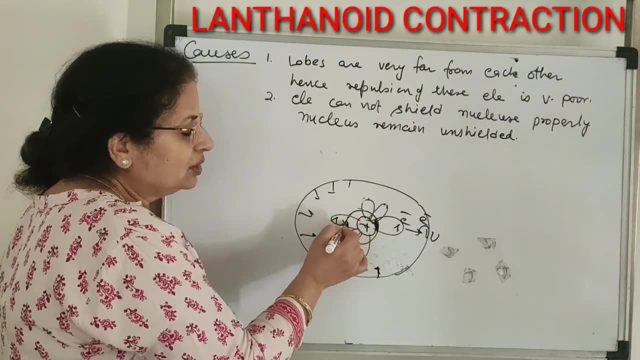 It will remain uncovered. It will remain uncovered, So it will attract the 4S, 5S, 6S electrons And when this electron will come here while moving, then what will happen? It will shield from this side, But it will not shield from the rest of the side. 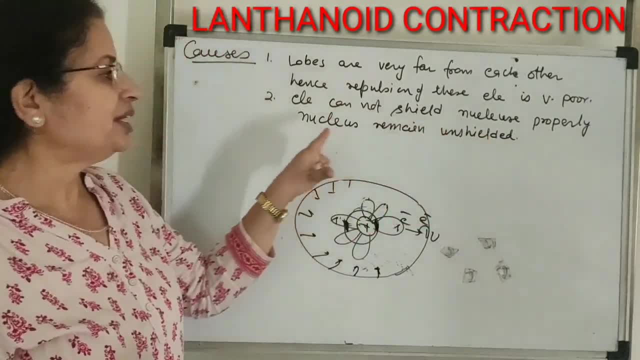 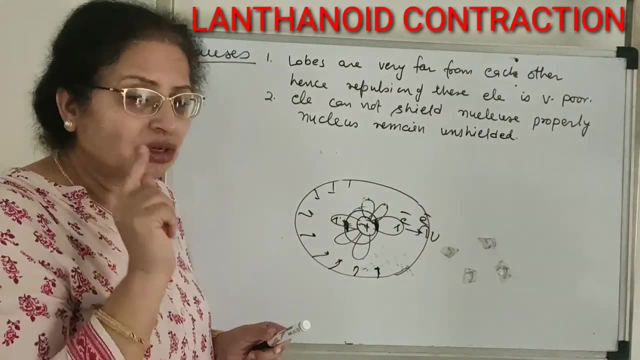 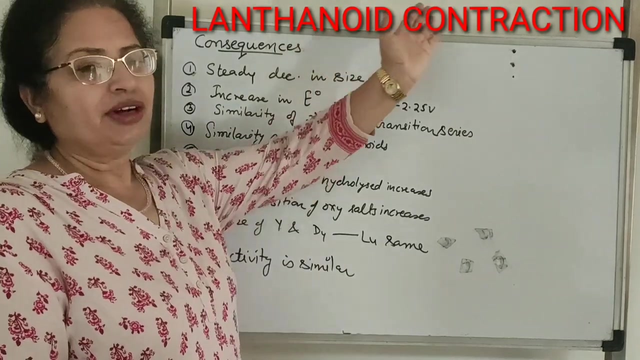 So we say: electrons cannot shield the nucleus properly. Nucleus remains unshielded. So these are the two factors of new lanthenoid contraction. Next is consequences of lanthenoid contraction. Consequences of lanthenoid contraction. What do we see in consequences of lanthenoid contraction? 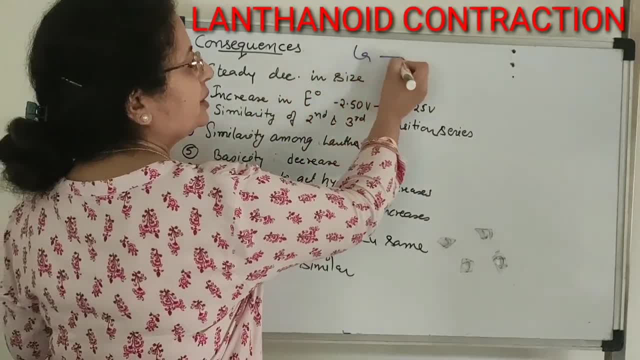 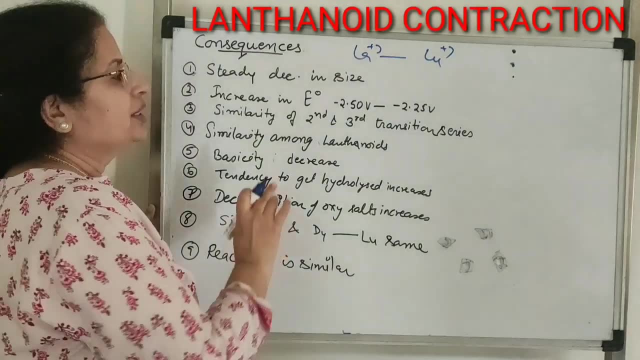 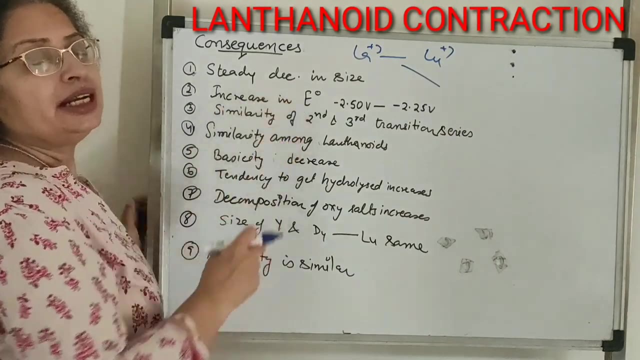 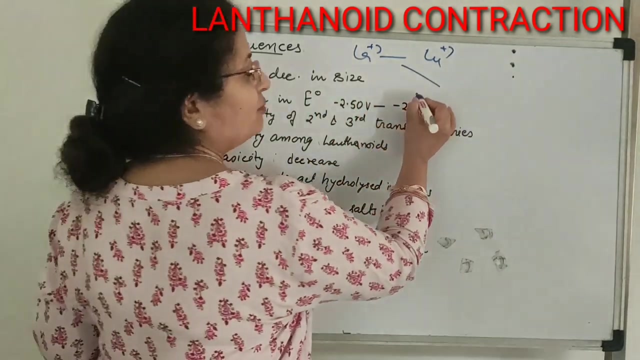 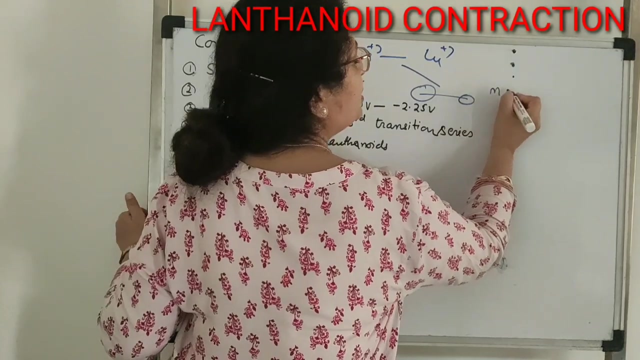 That throughout the series, which means lengthen on to plutetium plus 3.. The size is decreasing regularly, So we get the size in this way. Second, increase in standard electrode potential, Because size is decreasing left to right, so the value of standard electrode potential means 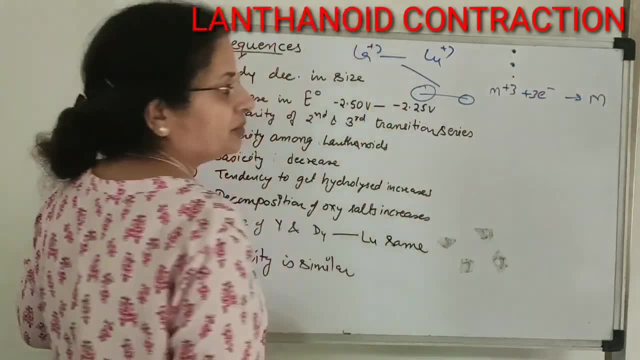 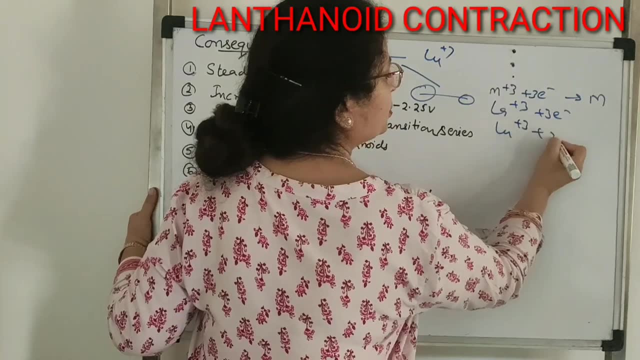 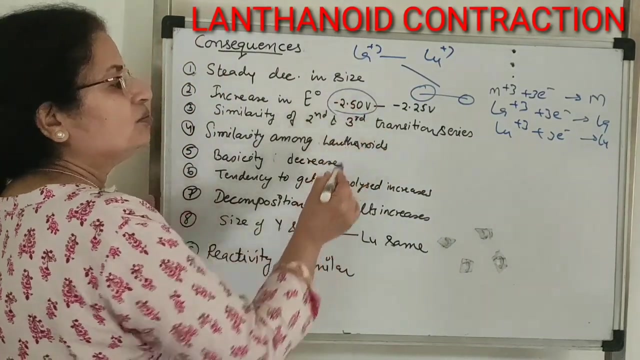 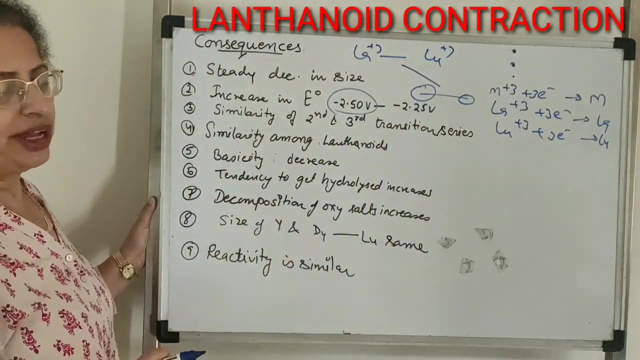 M plus 3, 3 electrons give M For lanthanum and for lutetium. both The value of this is: for lanthanum it is minus 2.50 volt and for lutetium it is minus 2.25 volt. 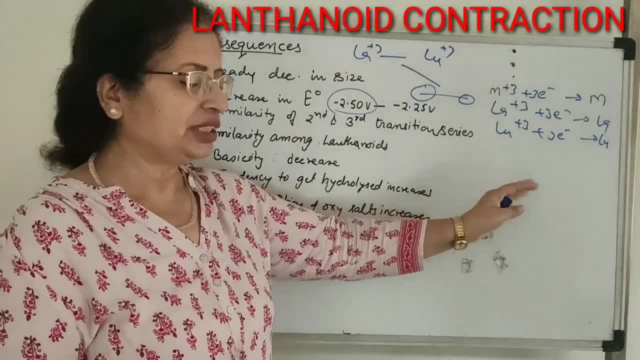 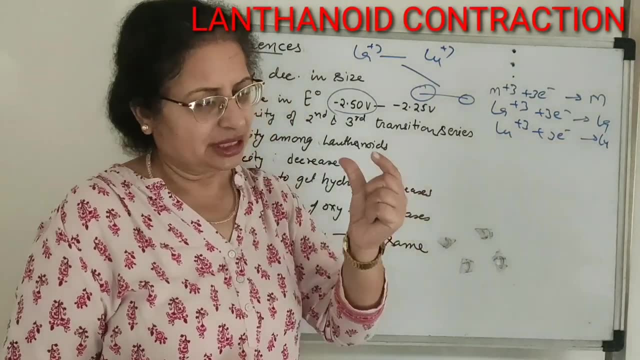 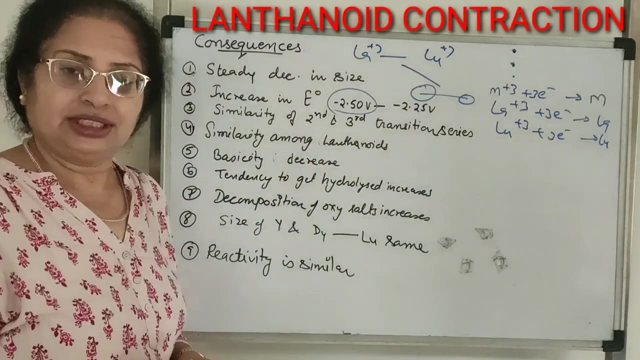 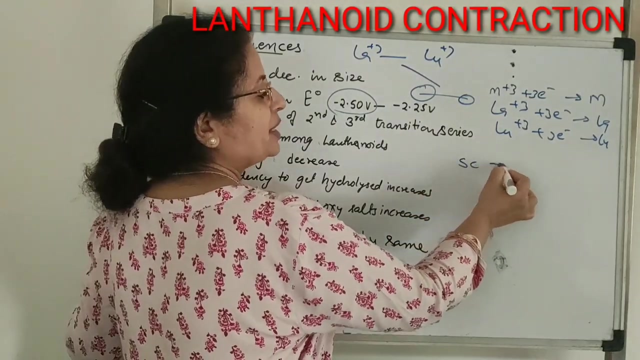 So it means the value of stentor electrode potential increases. It means it will easily reduce by taking electrons because its size is small. Then similarity of second and third transition series. Yes, it is very important consequence You see in this periodic table when you write scandium, titanium, vanadium. 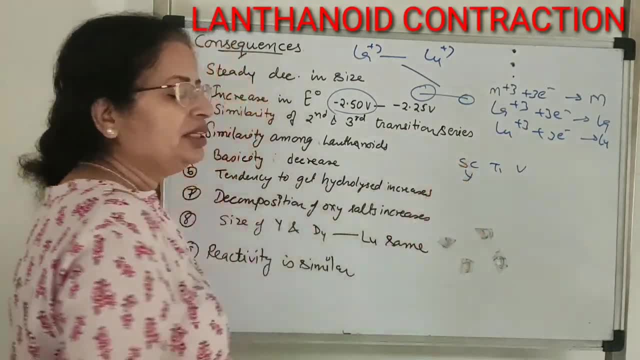 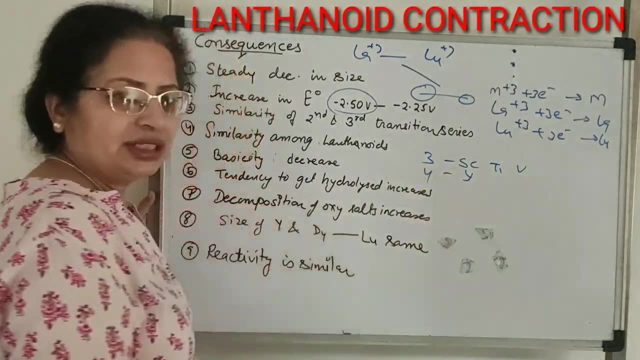 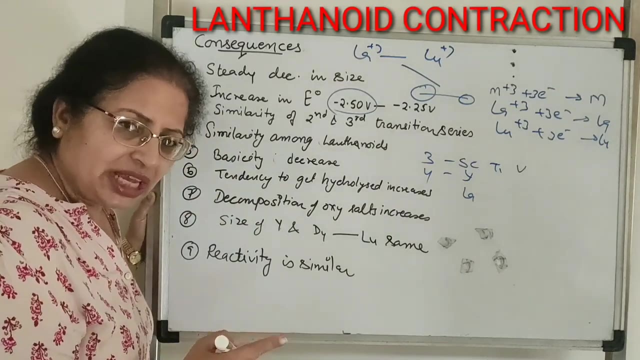 then here in third B, what do you write? below, scandium Yttrium, This is your third 3D series and this is your 4D series. Below yttrium comes lanthanum. So in any group, from top to bottom, the size increases. 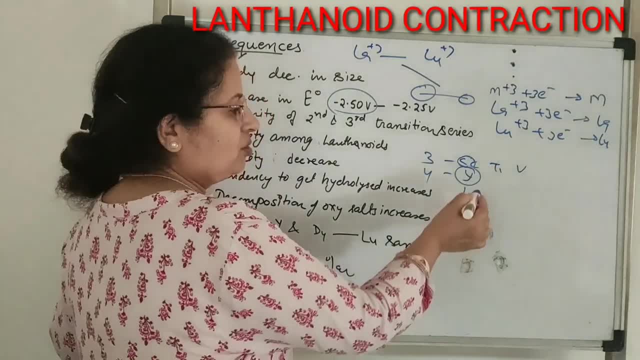 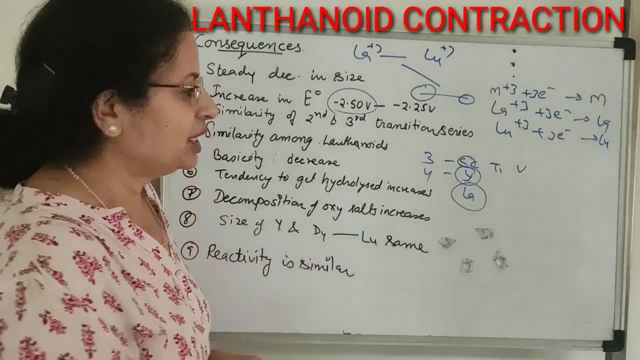 Because if its size is this much, then its size will increase and its size will increase. But what is the size of left to right? It decreases. So we had seen this lanthanum from vanadium to lutetium. 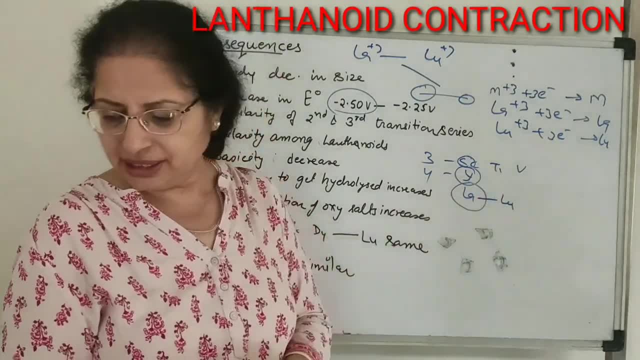 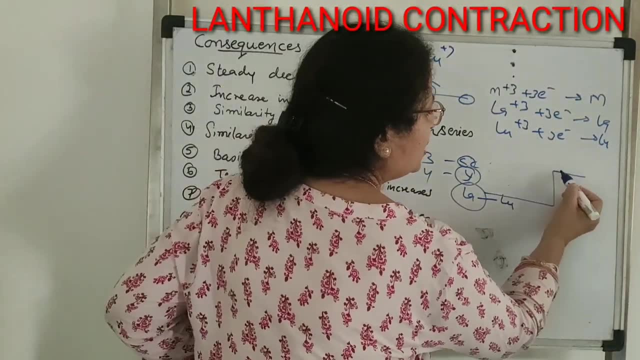 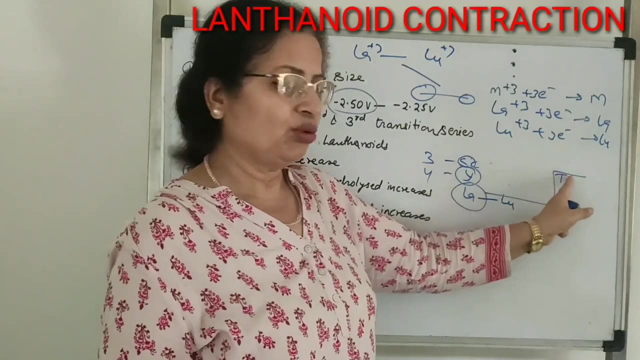 it is between these two. Scandium is not just above titanium here. Its position is after 14 groups here. So if we see scandium to titanium, then only one proton is increasing. One proton is increasing, so the size is decreasing a little bit. 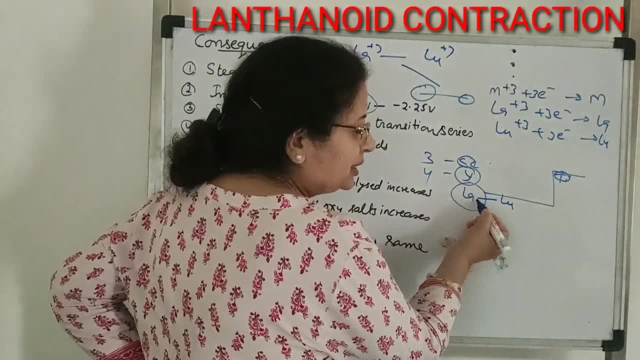 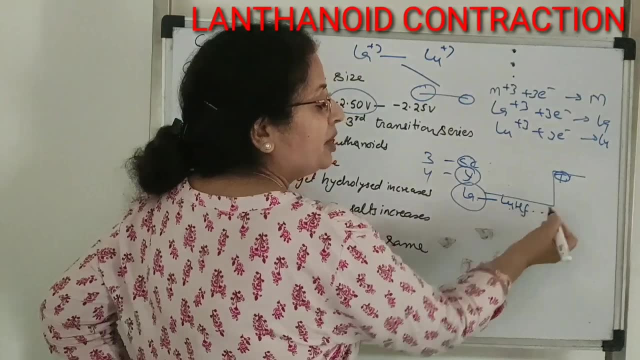 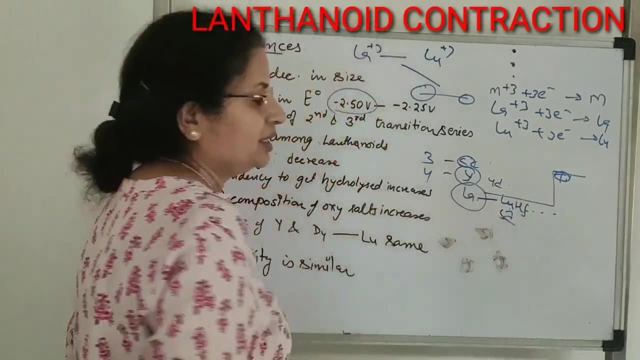 And the number of shells is equal, Whereas when you do lutetium from lanthanum, and then what do you go into Half-mium? After half-mium, you go further into the 4D series, And here this is the 4D series and this is the 5D series. 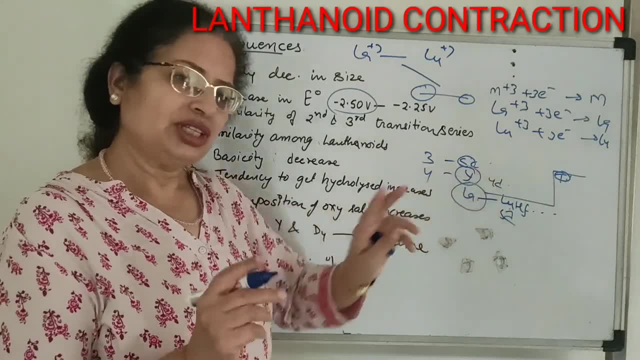 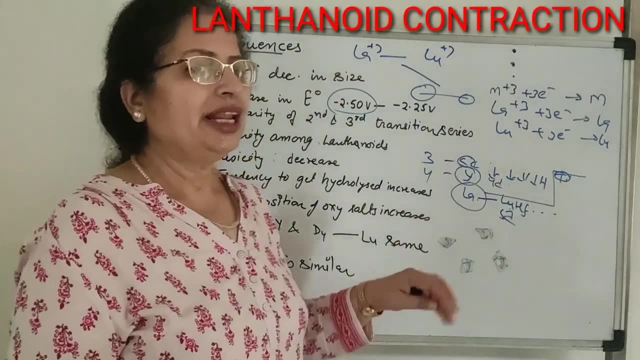 So what do you see? 3D to 4D. So the size is increasing. normally Like this, from here to here the size is increasing. Why? Because when it goes from left to right, only one proton increases. 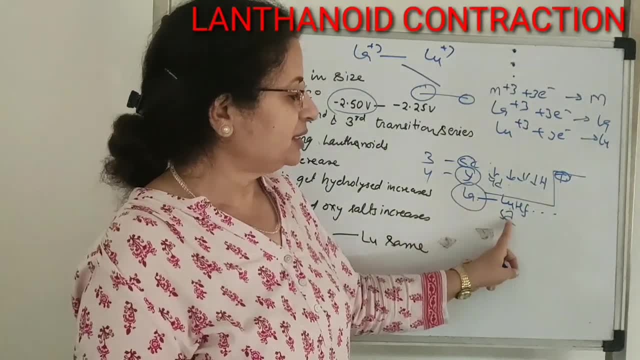 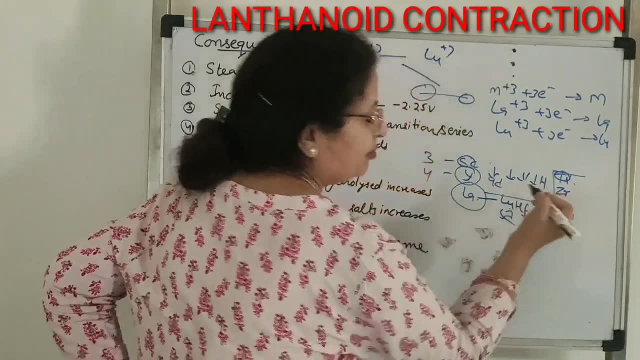 But as soon as you go from lanthanum to half-mium- and where does half-mium come? Titanium, zirconium, half-mium, It comes below this. So you see, from scandium to titanium, one proton is increasing. Yttrium to zirconium, one 39 or 40. But to go from lanthanum to half-mium, you have increased 15 protons. Its number is 57.. And what is its number? 72.. So these many extra protons contract the shells a lot. So the size that increased from here to here does not increase from here to here. Rather it decreases slightly Or it remains the same. Either it is equal to it or it decreases slightly. 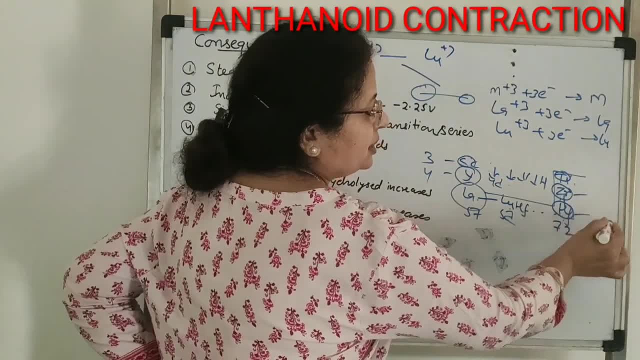 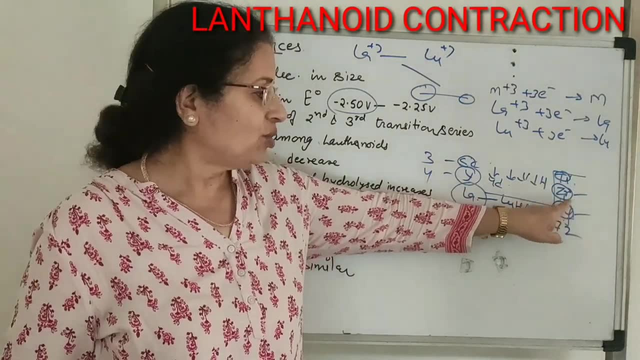 So what do we see? This 4D series or 5D series? Similarities come in both. It does not come in 3D and 4D. Why? Because the size is increasing, But it comes in 4D and 5D. 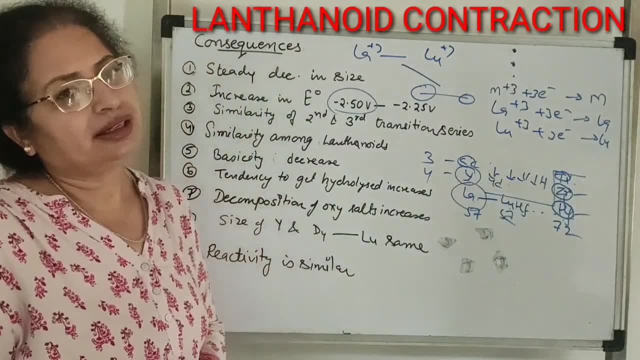 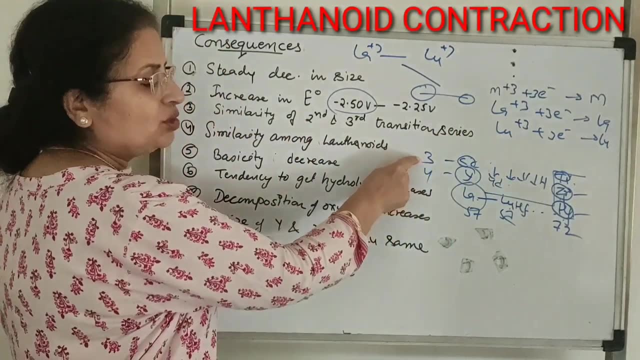 Because of lanthanide contraction, their size is the same, So this was the similarity of second and third transition series. This 3D series is called first transition. We call 4D first transition. We call 4D second transition. 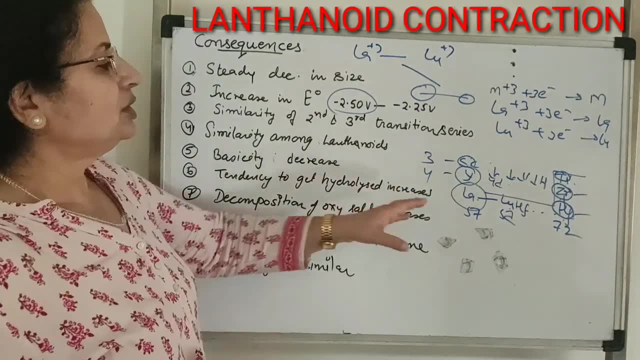 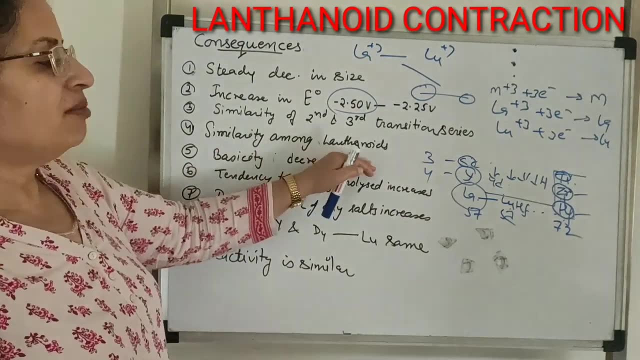 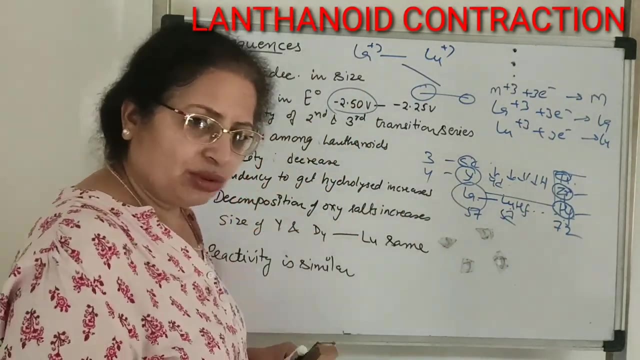 And we call 5D third transition series. So that is why similarity comes in second and third transition series. Next is similarity among lanthanoids. So when their size is almost the same, it is decreasing slowly. So whatever properties are there, 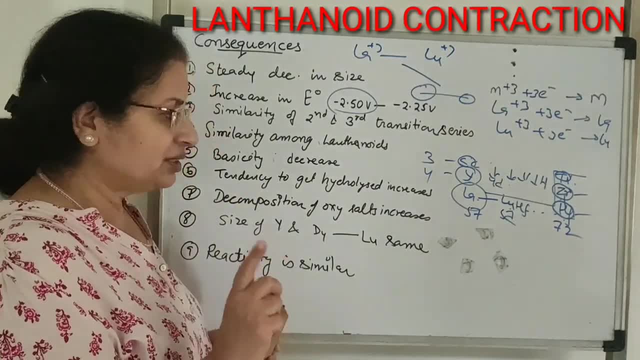 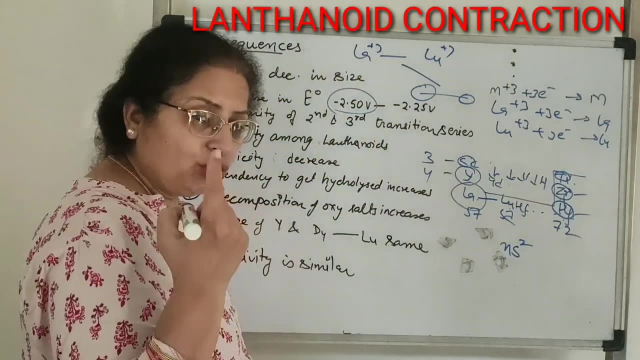 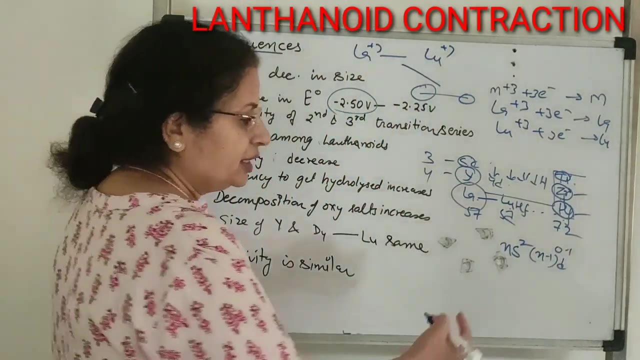 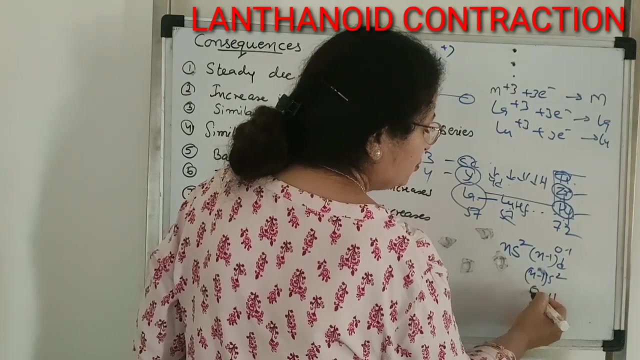 ionization potential, electron negativity: they do not decrease much. Secondly, their outer most shell configuration is same NS2.. And inside that of penultimate N-1 DS2,, N-1 S2, and N-1 P6.. 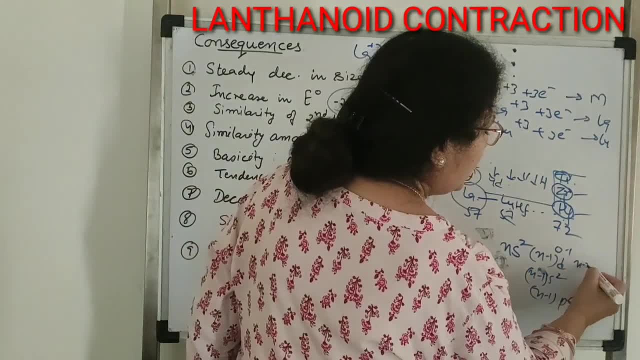 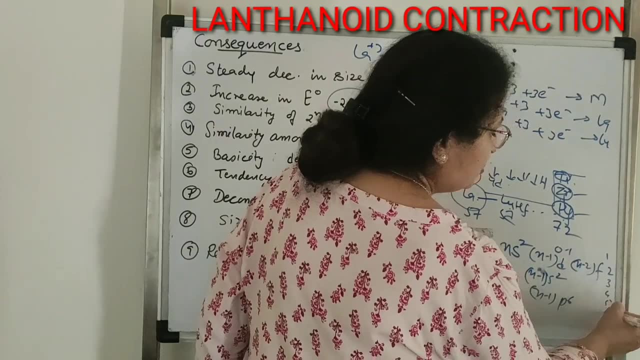 Penultimate is same for all, But N-2F is anti-penultimate, Only this is changing, Sometimes 1,, sometimes 2, sometimes 3.. Sometimes 4,, sometimes 5,, sometimes 6.. So it means: 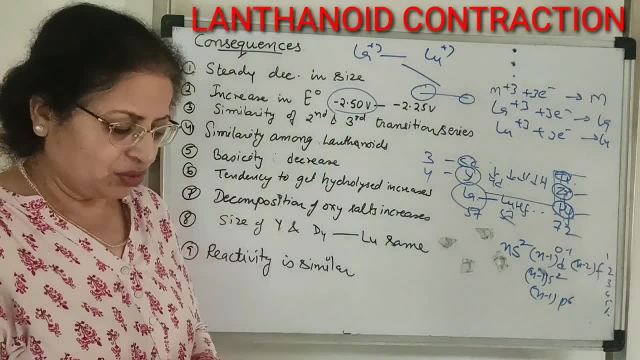 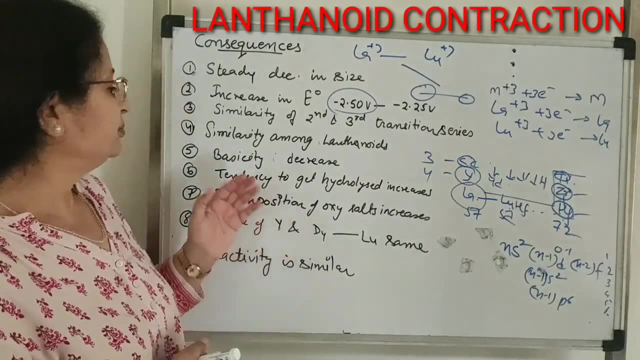 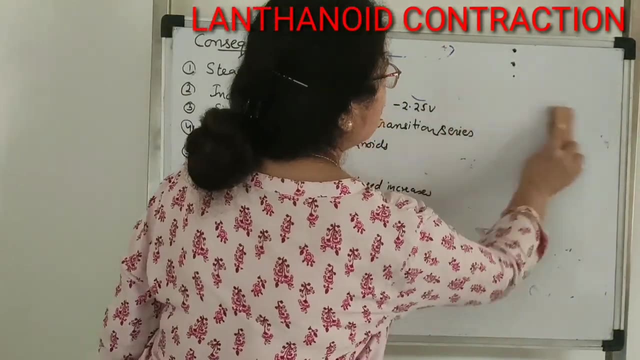 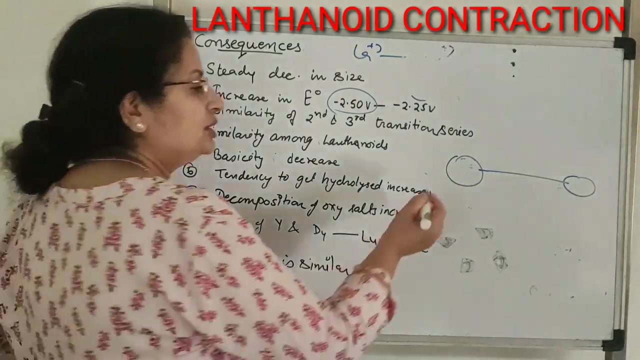 outer most. two shell's configuration is same, So their properties are same, They behave the same. Basicity decreases. Why does basicity decrease? You pay attention? Because left to right what is happening- Decrease is happening. So when 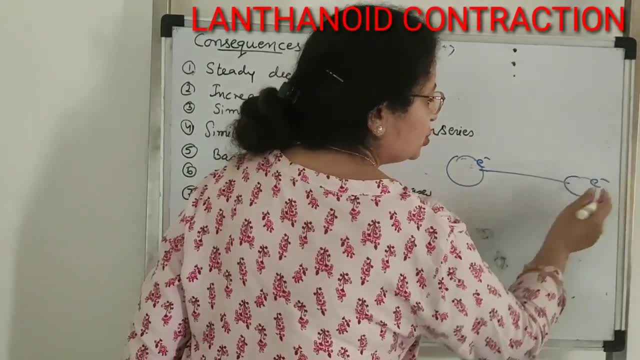 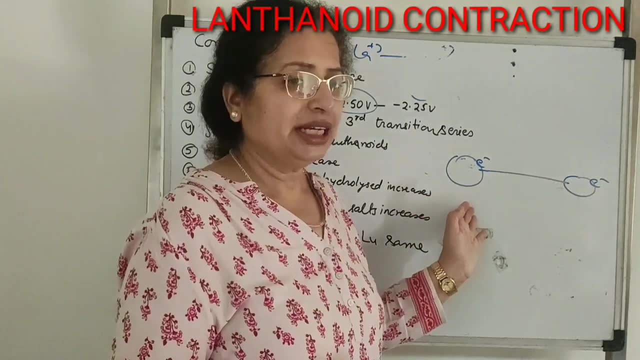 this electron is given to someone and this small electron is given to someone. Basicity means donation of electron, To give electron easily. So tell me, this one will give easily or small one will give easily? This one will give easily. 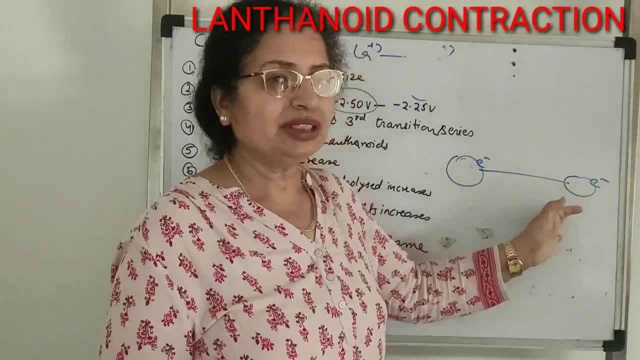 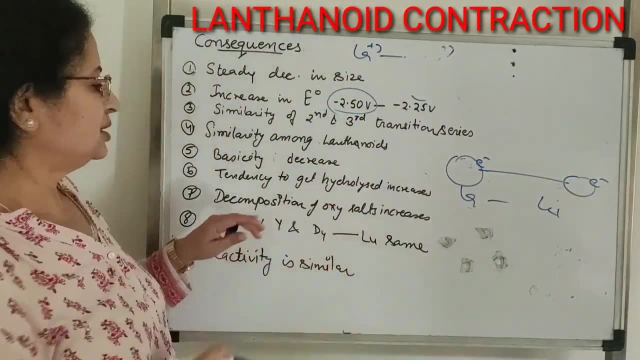 It means its basicity is more And the basicity of lutetium is less. So you can say: from lanthanum to lutetium, basicity decreases. Next is tendency to get hydrolyzed increases. What does it mean? 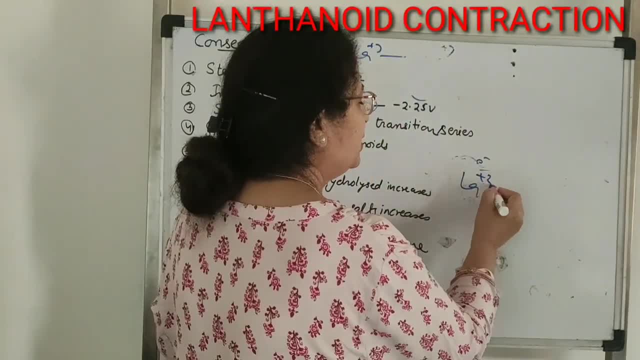 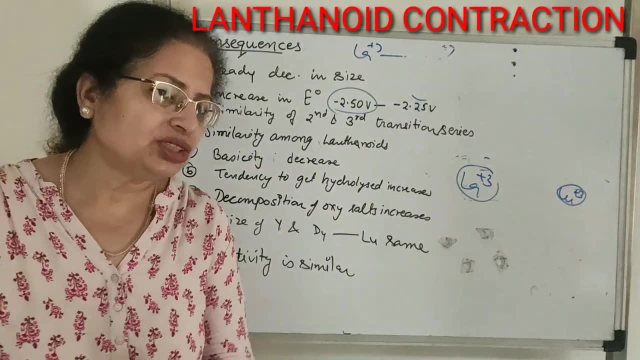 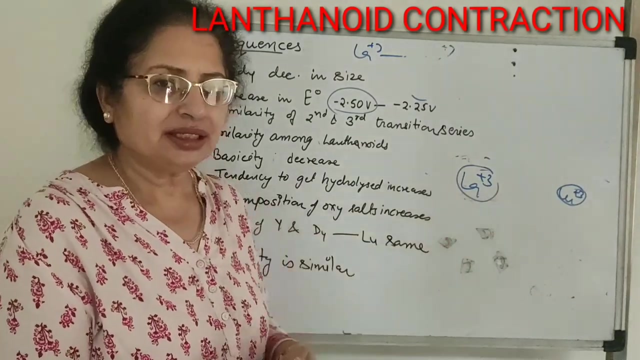 That you took a lanthanum plus 3 ion and this lutetium plus 3 ion. On both of them you can see the size. Its big and its small. Charge: same Plus 3, plus 3.. So charge density. 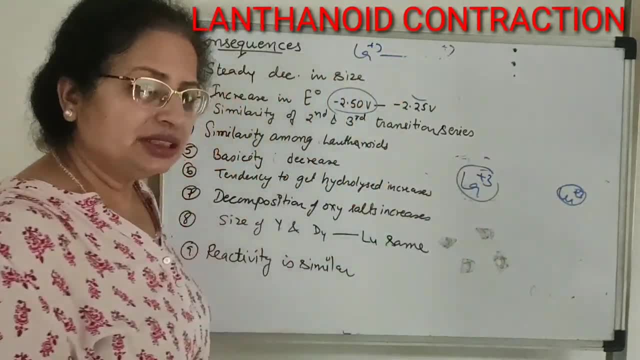 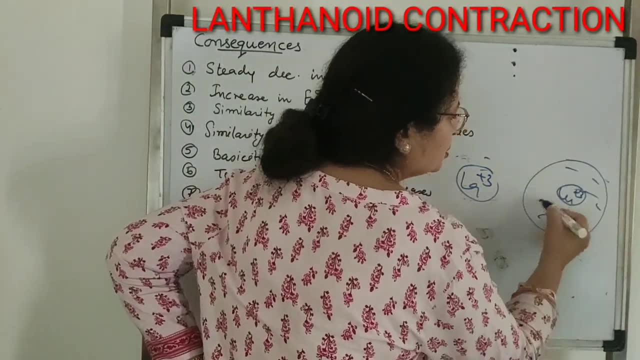 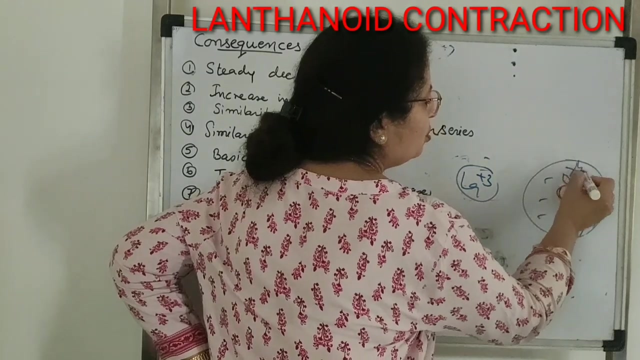 What will be of this Less? What will be of lutetium More, When its charge density will be more then around it, water molecules, OH, H, O, H, H, O H H. What will happen in this way? It will increase a lot. So its hydrolysis, or to get hydrolyzed its tendency, will increase When its charge density is less then around this much, only water molecules come Next. decomposition of octane Oxi-salt increases. 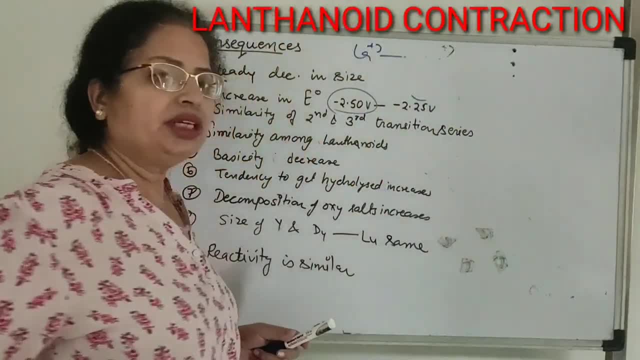 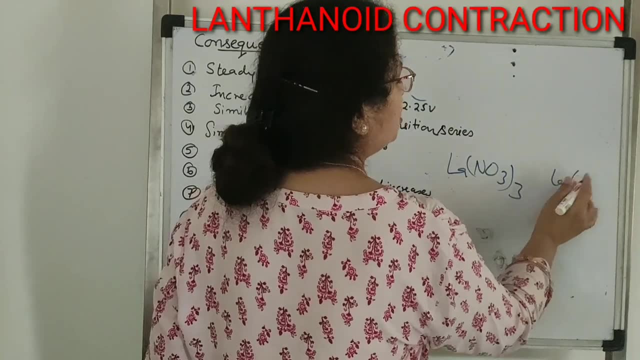 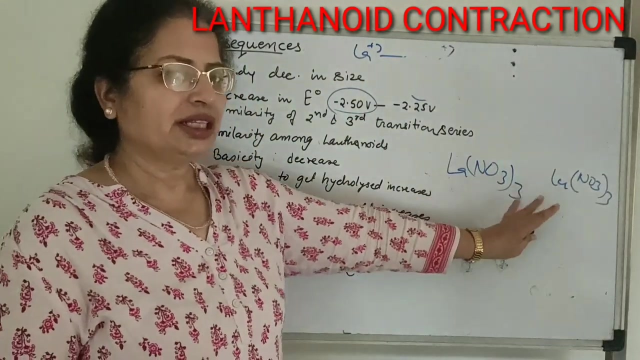 Now, decomposition of oxi-salt increases, means, you see, as this lanthanum is nitrate and this lutetium is nitrate, Lanthanum to lutetium, This is its oxi-salt in a way, because it has oxygen. 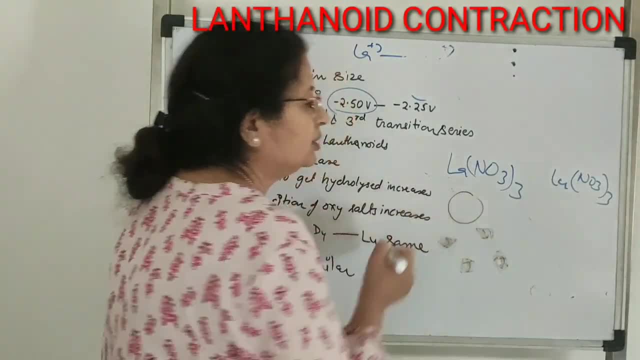 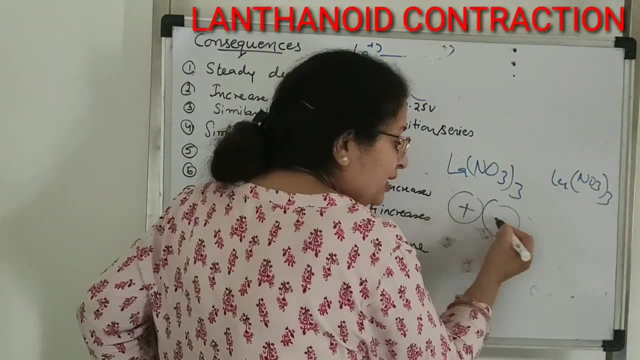 The size of lanthanum is bigger, Bigger And the size of nitrate is also bigger. Why? Because 1 nitrogen, 3 oxygen, Bigger, So bigger cation and bigger anion. What will happen? Stable. 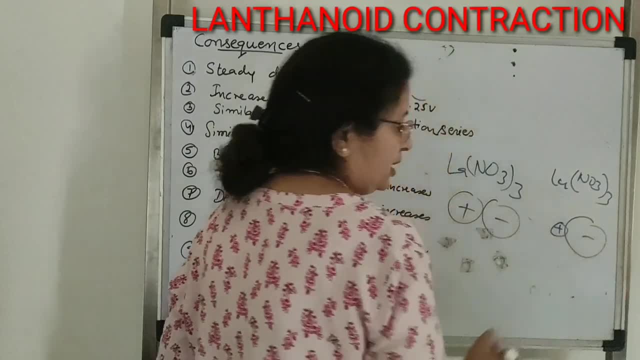 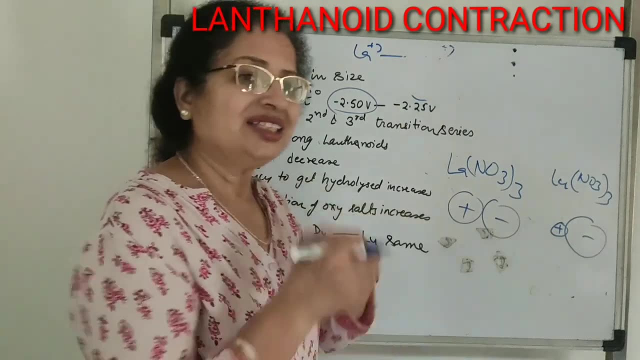 But small cation and bigger anion. What will happen? Unstable Lutetium is small. When it is unstable, then it will decompose easily, And by decomposing means at low temperature, only by decomposing. 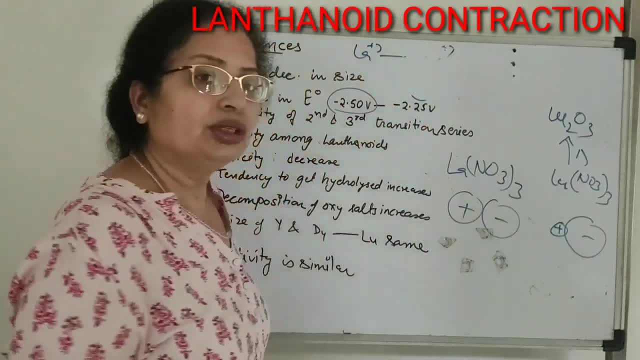 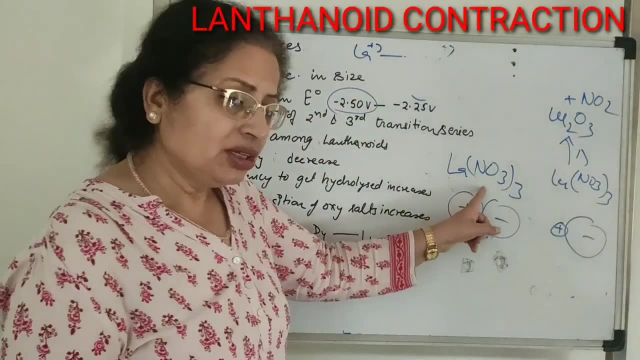 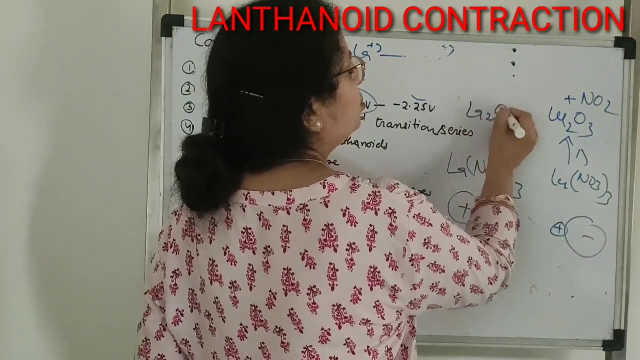 it will give LU2O3.. Lutetium oxide plus nitrogen dioxide. But this will also break in this way Lanthanum If we heat it: LU2O3, Lanthanum oxide plus NO2.. But 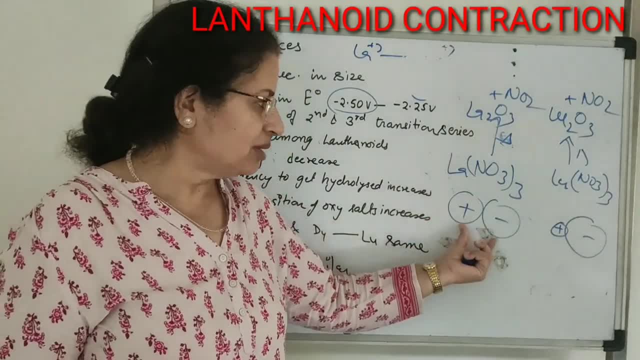 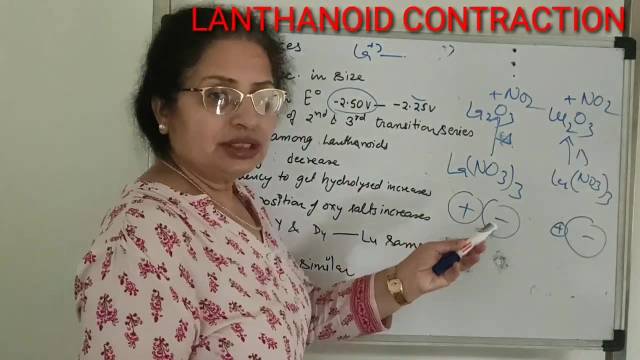 what will happen? It will happen at high temperature because it is stable And it will break when it is heated a little. So this was: decomposition of oxi-salt increases Means. it increases easily. Next is size of yttrium. 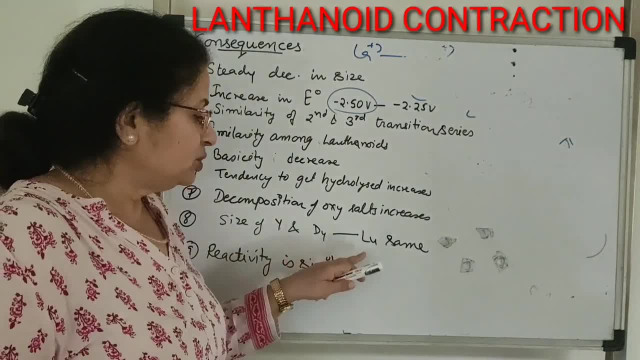 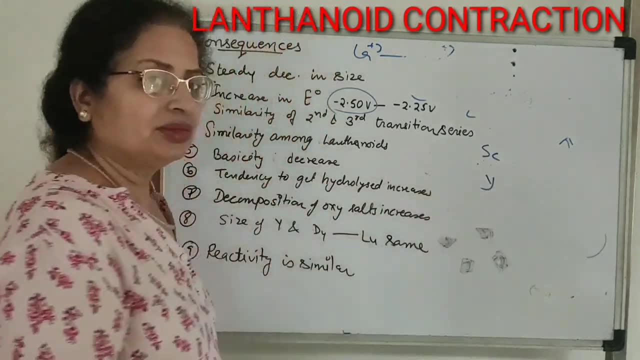 and dysprosium to lutetium is same. Again, very interesting Because what is below scandium Yttrium, Below yttrium is lanthanum And you know size top to bottom increases. 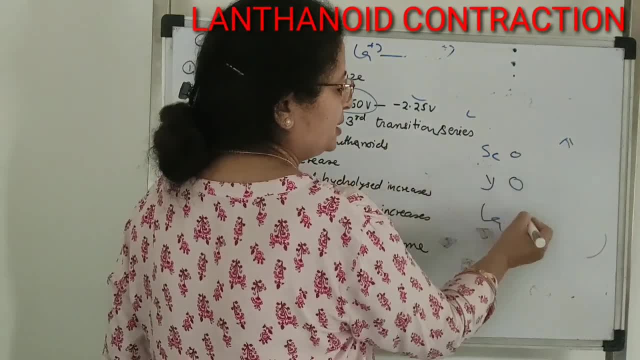 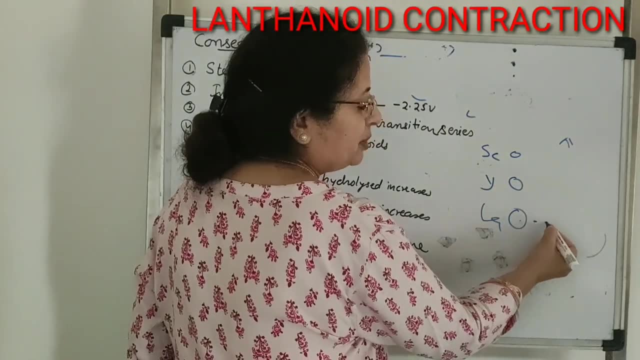 So I made their size increasing, But what is left to right Decrease. So I went from lanthanum to cerium presonate, cerium presodymium, neodymium promethium samarium.